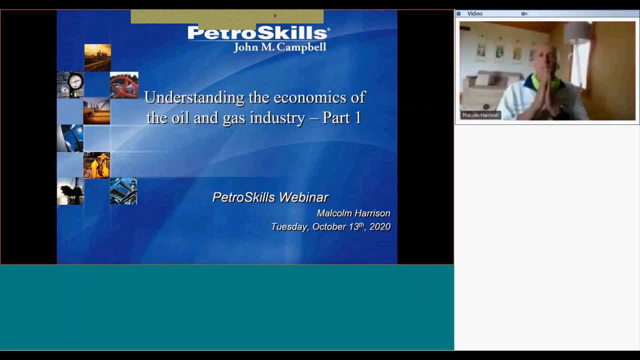 two and maybe three. But before I talk about economics and prices and numbers of things, I figured it's probably a smart idea to introduce myself. looking down the list of names of attendees, I recognise a few but not all. So I am a firm believer that the best teacher in life 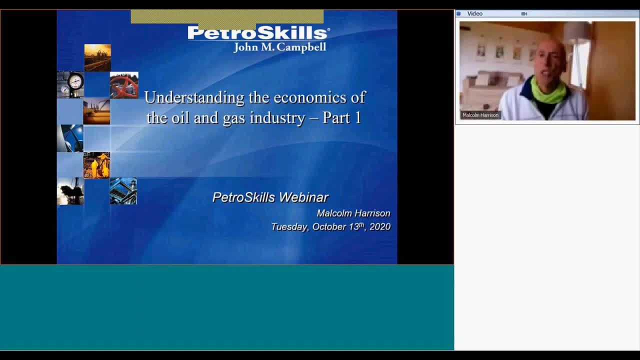 is failure. There's nothing better than making a mistake from which to learn, And my claim to fame would be: I have been making mistakes in the oil and gas industry for the last 40 years. I hope this next slide will give you some idea of just how well life has taught me. 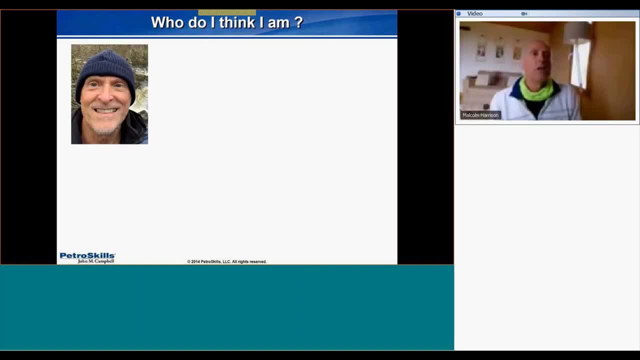 So here we go. Who do I think I am? Who do I think I am? This is me. This was a picture taken back in February of this year in Aberdeen in Scotland. As you can see, a bright-eyed mid-30s, late-30s sort of guy making his. 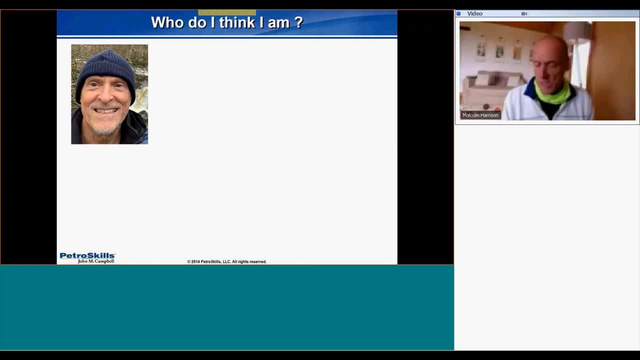 way in life. And then, of course, right about March, in this part of the world, the world came to a close, And this is what I look like today. Here we go. You know, I thought, as I posted that picture, if I 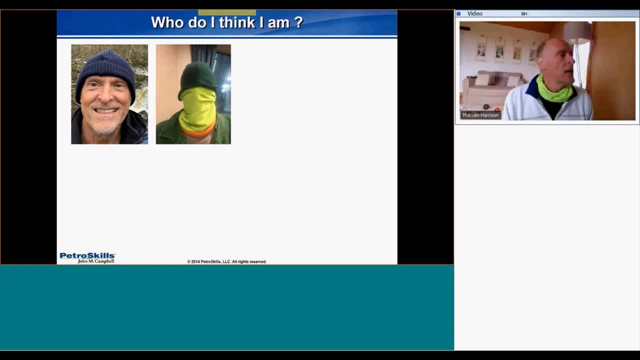 walked out on the streets looking like that a year ago, I probably would have been arrested as a potential bank robber. Today I'm seen as a fine, upstanding citizen because I'm fully clad, Such as. the world changed in six months- And had it not changed, I suspect I 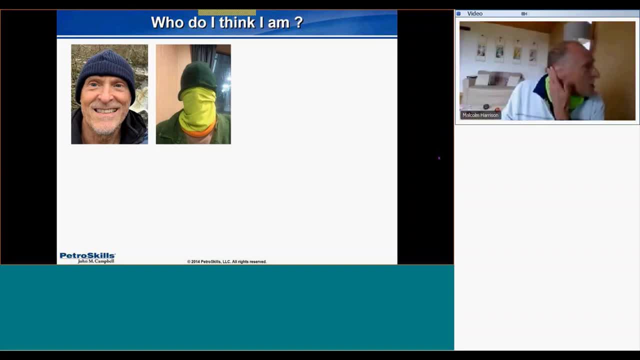 wouldn't be talking to you on webinar. Anyway, that's what I look like. This is where I started life, or started work at least, with these guys. You've probably heard of them, BP a very long time ago Now. one of the things BP recognized very quickly after joining them was my 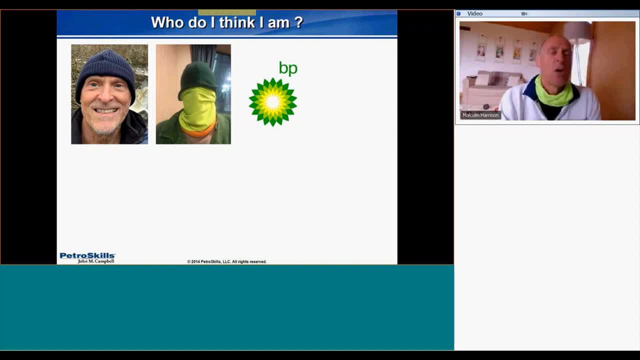 desperate need for education. They packed me off to university to do a chemical engineering degree. So I was a chemical engineer in the early 80s from the great University of Bradford. Many of you are going to be too young to remember 1987. But in 1987, the world stopped. 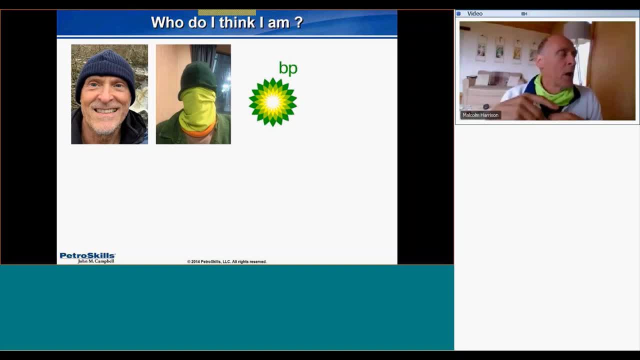 much as it has in 2020,. at that time, because the stock markets of the world collapsed, the world GDP collapsed and the oil price collapsed. Oil dropped about $10 a barrel And BP very generously offered people a suitcase full of money. 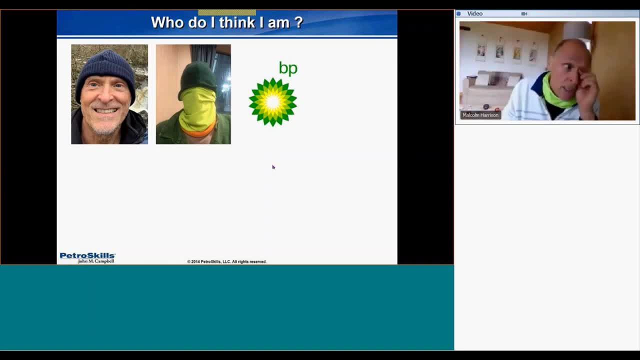 in order to leave the company, And so I duly departed, armed with my suitcase, and I joined this company. BOC stands for the British Oxygen Company, who no longer exists- made their money from cryogenically turning air into oxygen and nitrogen. 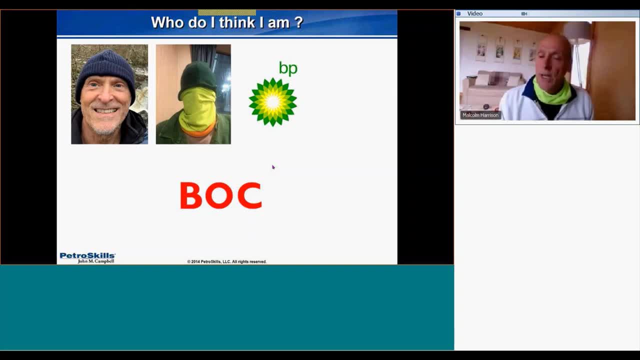 and various other rarer gases. BOC too, recognized my desperate need for education, very kindly showed up to the UK. I got an opportunity. I actually went to university for two years to do an MBA And I emerged two years later to join a team of people whose responsibility 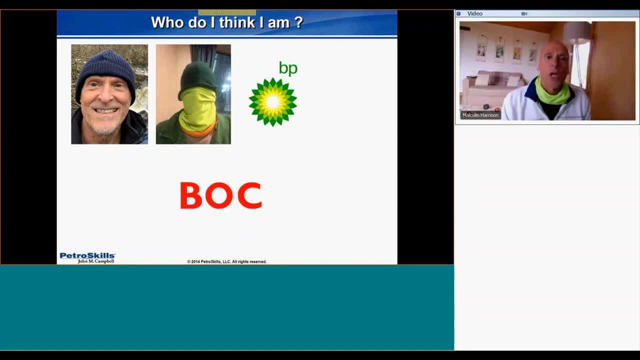 was to prepare the company for the future. We developed a new range of products, a new range of air separation plants, which were so good that we sold a dozen of them, but actually were so bad. and shortly after that the VOC share price crashed. VOC was taken over by a German company. 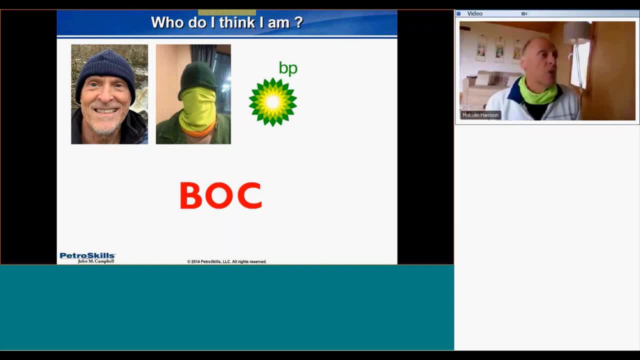 Lindy and VOC offered their employees in return for leaving a suitcase full of money, and so I departed VOC after 10 years- so we're probably up to about the year 2009- and I joined this organization. this organization is Foster Wheeler also no longer exist today. were 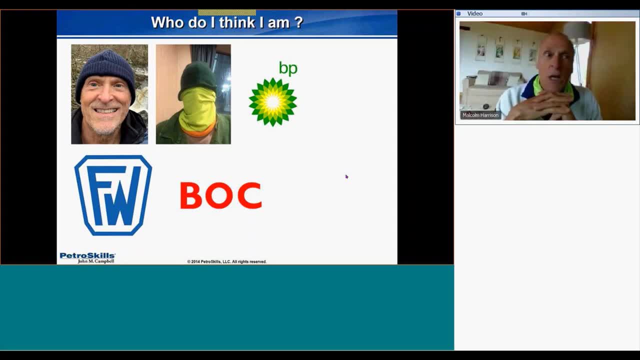 an EPC contractor were at one point a very successful EPC contractor and possibly- and I am proud to say that I was part of the senior leadership team that successfully drove Foster Wheeler into the ground and reduced the share price to the level where AMEC stepped in and and and took them over. I think you might be starting to see the pattern of failure. 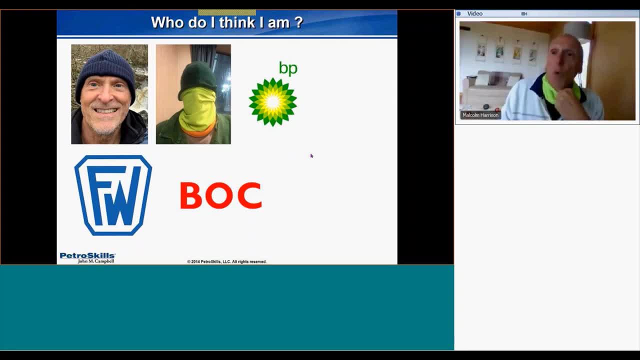 that I talked about on the previous slide. so for Foster Wheeler, I joined a company called BG. BG no longer exists today. I was BG's chief process engineer and clearly was getting better at my art, because I managed to turn BG around in five years and the collapse, the share price and BG were taken. 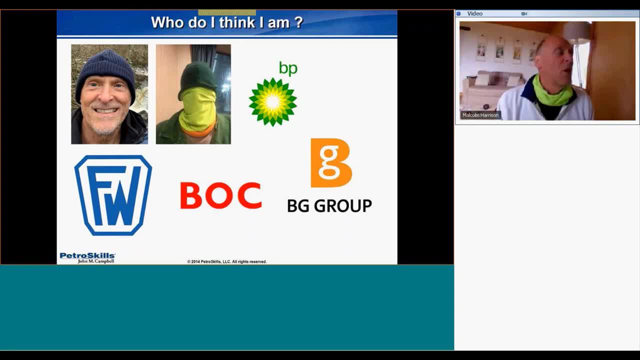 over by Shell. the, the office facility in which I was working was that was was closed and BG offered people a suitcase full of money in order to leave the company. so now the proud owner of three suitcases. I had enough suitcases in order to to retire. find retirement to be very dull. 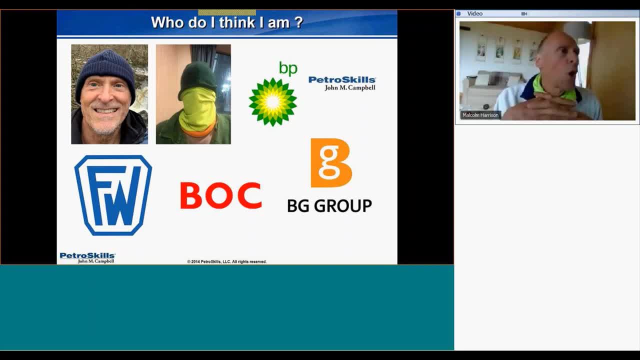 and I took a call one day from an old colleague in Petroskills, John M Campbell, and I joined as a, as a teacher, six years ago. I passed along my AIM and shortly after I graduated the well, I've just put something in here as well, in kind of on. recall myself a mumunhut, as I said, but find retirement on three. 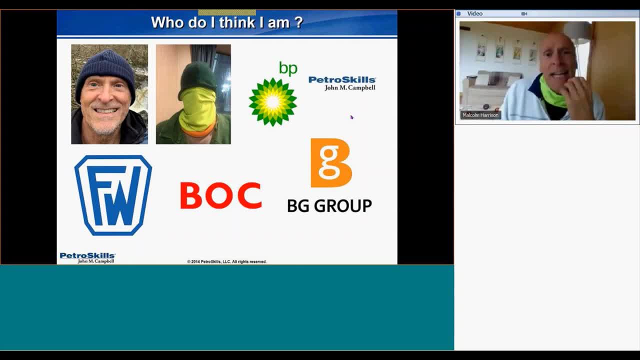 suitcases and if you add that in, I think would fetch about five percent, I assume, of some uh really was invested over eight hundred dollars and it told me actually it was a three select two, so not a good way to go about that, but once I started to fill that out it really helped me. 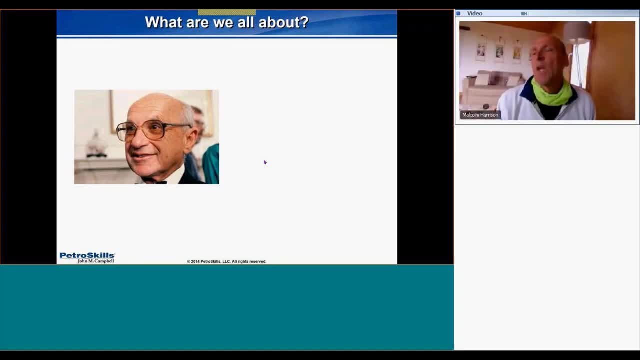 who knows who this is and of course your microphones are all muted, so you can't respond to the question. you can probably chat about it, but i'll give you the answer. this is a gentleman called milton friedman. some of you may have got the answer: milton friedman was a 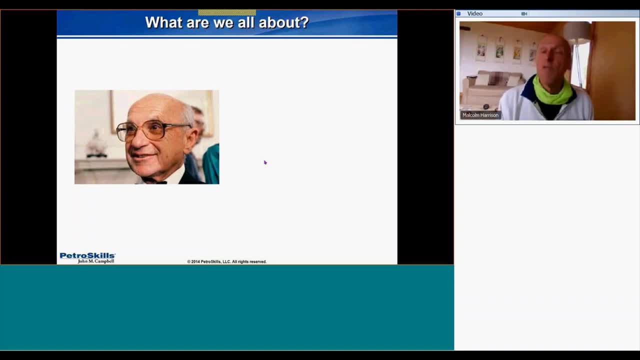 a very well-known, renowned even- management consultant and management philosopher, uh, even back in the 70s and the 80s, uh, and many, many responsible for many, many quotes, but this is the one that i wanted to use to set the scene for today, so sometime back in the 70s. 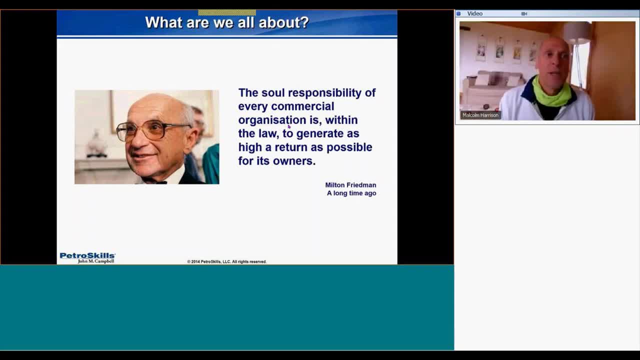 milton friedman said: the sole responsibility of every commercial organization is, within law, to generate as high a return as possible for its owners. many people have disagreed with that statement. personally, i quite like it. it for me, it means that every single one of us who are working for a commercial organization um bear that responsibility. 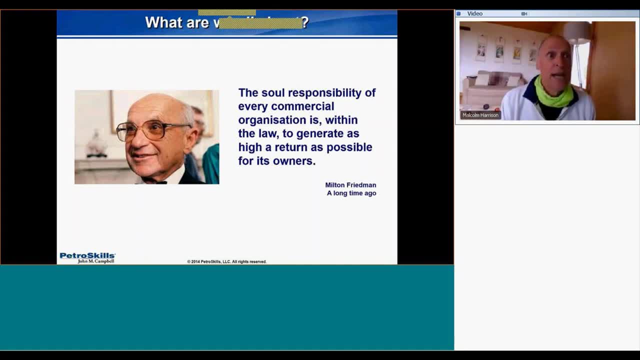 to return as higher return as possible to our own, sometimes, to shareholders, to pension funds, private equity companies, to individuals. um, the reason i put the reason i put the quote up, is that it's not just a quote, it's a statement. it's a statement of it does mean that those of us engaged in whatever part of the chain we're in in the world of oil and 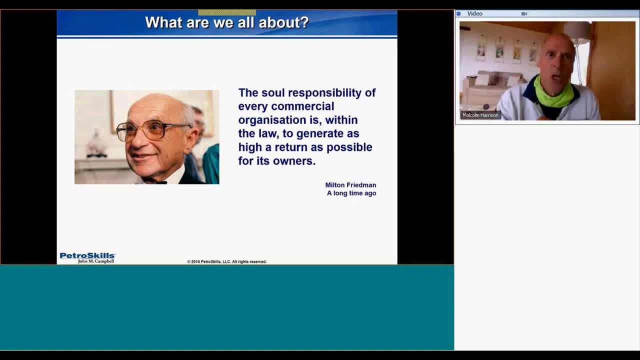 gas, have some responsibility to understand where the money is, where the profits are and hence what it is that we have to do, what our part is in generating that, uh, that high return. so that was my setting the scene. i wanted to, i wanted to hop to um. 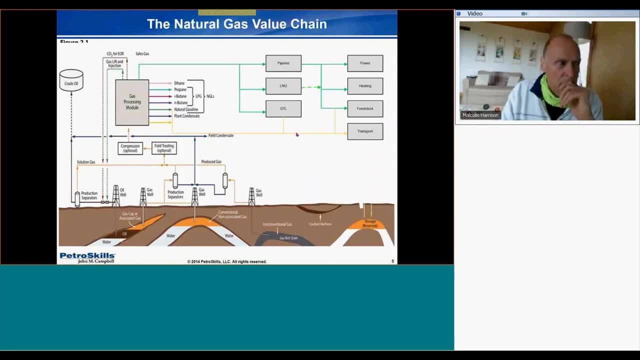 the next slide, which is just, which is a single picture, and in it's a single picture that is trying, and does not a bad job, of summarizing an entire industry in one picture. so remember the: the goal is to make as much money as we can. we make that money by extracting, 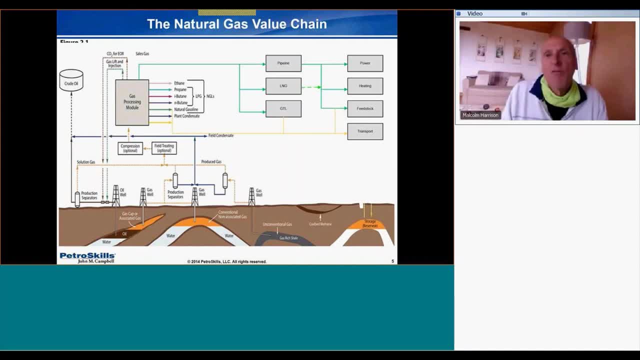 hydrocarbons from the ground. we remove the stuff that can't be sold- stuff like sulfur, stuff like, occasionally, carbon dioxide, stuff like water- and, from the bits that remain, we process them to make as much money as we can for their components, as, as is possible, lots and lots of the of the of the money and the value is driven by. 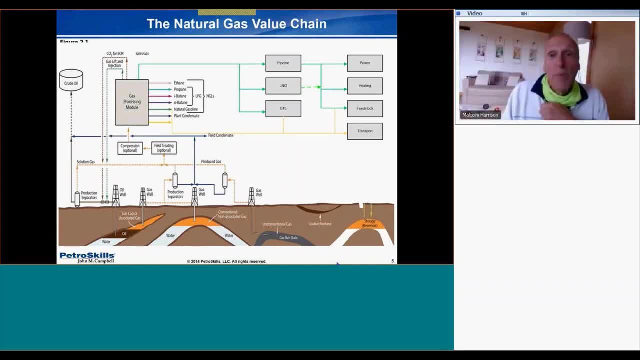 what's underground, how it got there and how best we are going to exploit it. i'm not going to talk about that. that is part three. if we get to part three in this uh, this, this series of uh webinars, um, what i am going to talk about is the stuff above the grain. 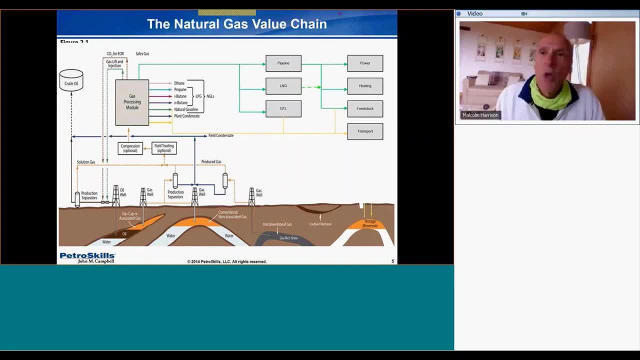 and essentially we're off. we're known as the oil and gas industry and predominantly what we produce is is oil and gas. you'll see here we've got our little gas processing module with sales gas coming out of the top. it works its way to a market in one way or the other, maybe via a pipeline, maybe if the market 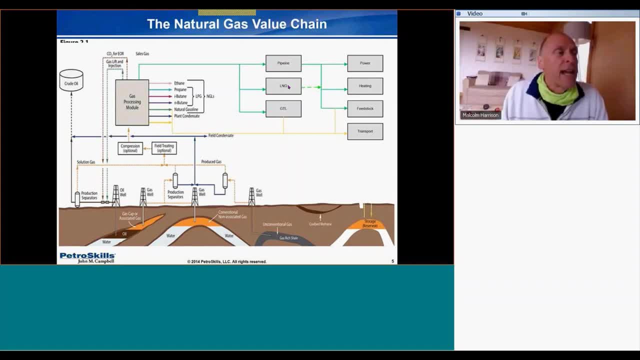 is a long way away by being liquefied and shipped and regasified and largely gas feeds. three separate needs, three separate consumer blocks, customer blocks, industry sectors. one, the generation of power. the second, heating, be it of domestic properties or commercial properties. and the third as a an industry feedstock. an industry feedstock where it's used to generate. 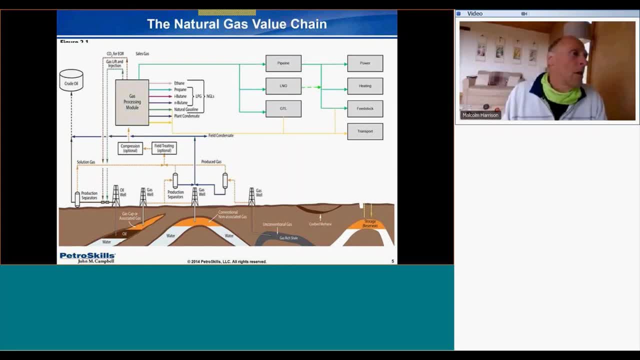 ammonia, hydrogen, methanol, petrochemicals and a range of of other products, and that's mostly where the gas goes off the bottom. here we've got, with the orange, the orange line. here we've got oil, oil which mostly goes to the transport sector, but the trains, boats, the planes, the cars and the 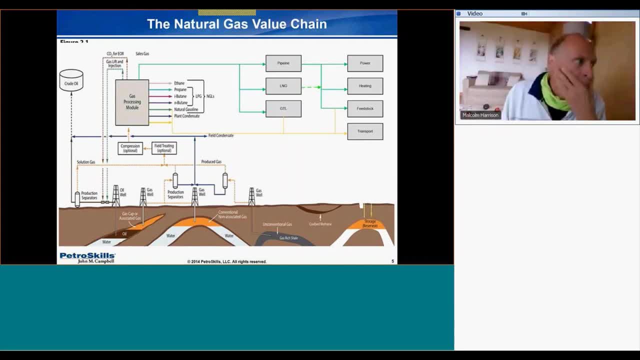 ships. i've already painted ships twice, though, and some too, going into feedstock- a minor way, which is to kind of put quantities into into heating and into into power. there's very little crossover between the gas and the oil. one of the ways in which we cross over is is the use of gas. 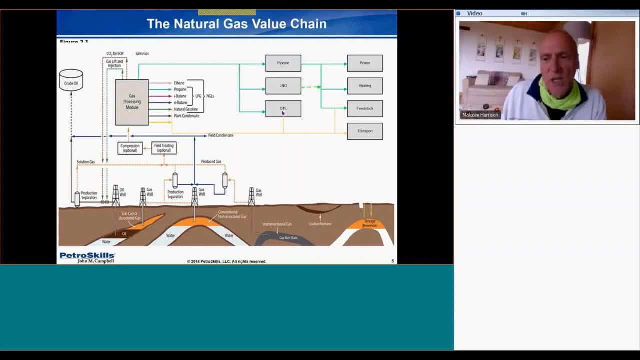 to liquids, uh technology, um, which essentially takes a gas feedstock and produces a diesel or a gasoline, the transport fuel as a, as a product. um, there are only four um gtl plants in in the world, And all there for rather specific geographic or political reasons. maybe 1 or 2 more, I think. I did see that Uzbekistan has just announced financial plans for developing the GTL plan, but fairly small in terms of their influence over the overall market. 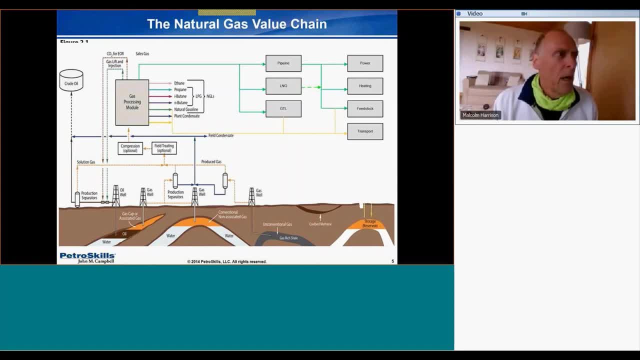 But there we have the industry in 1 single picture. When I was putting this together a couple of days ago, I discovered some numbers that are found to be quite useful. If you look at energy consumption in each of these 4 sectors, approximately 40% of the energy consumption is in. the section is in power. 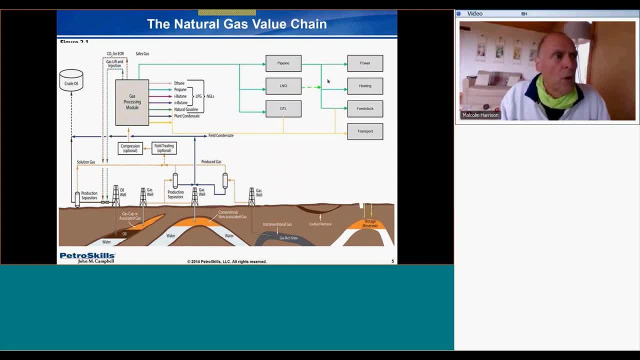 Now that includes coal as well as oil, although not nuclear, but hydrocarbons. so approximately 40% of the hydrocarbon usage is used for power and approximately 20%- But each of the other 3 blocks- for heating, for feedstock and for transport. 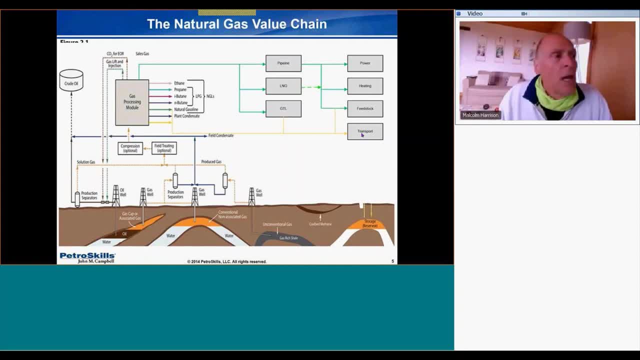 So there's a nice easy numbers to remember. The other number that I liked, which was quite easy to remember, is that 80% of the carbon emissions from these 4 industries are generated by the top 20 countries. So there's lots of 20s and 80s in that. 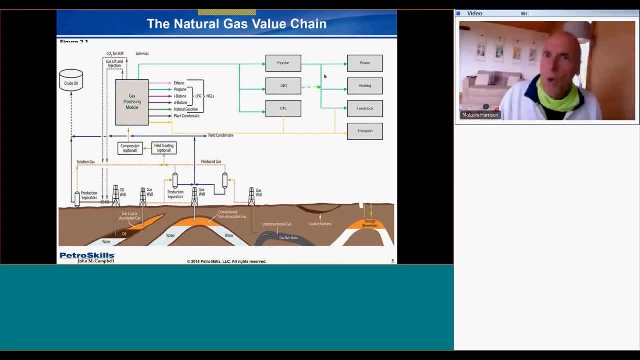 But look, but that's, that's the. we're the oil and gas industry. We produce, we produce gas, we produce oil. What's all this stuff in the middle? So, as well, we have the facility to produce ethane, to produce propane butanes. 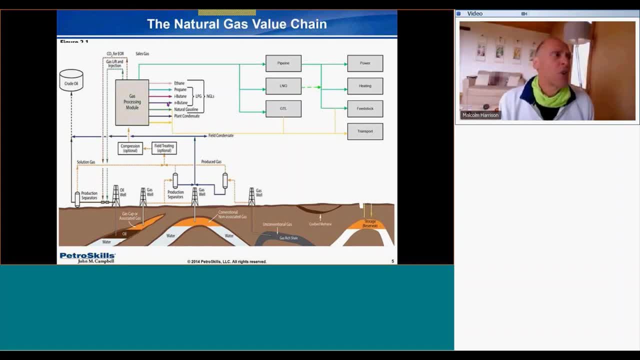 MGLs, which are essentially light oils, which goes straight into a gasoline feedstock. And the question is: why do we do that? Why do we produce these extra Byproducts? and I would suggest we do it for 2 reasons. For 1 of 2 reasons. 1 reason we do it Is because we have to, ie we have to- take light components out of an oil, because we've got to be able to transport it and it needs to meet a paper pressure specification. 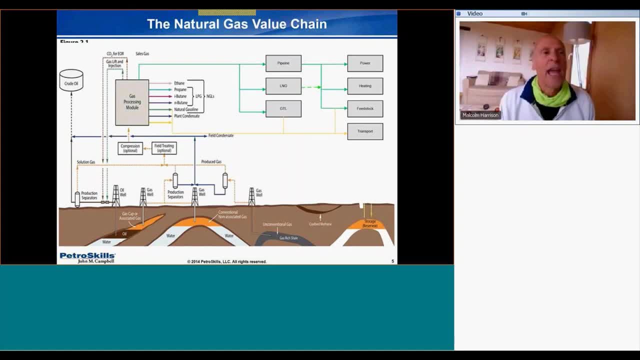 We have to take heavier components out of the gas Because it has to meet a heating value and it has to meet a dew point specification. So 1 reason we take them out is because we have to. But the 2nd reason is because we want to. 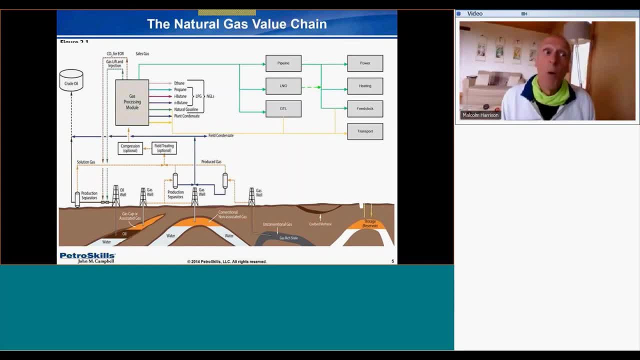 And in some cases we want to because we can make more money from selling them as individual components Than we can from, say, letting them slip into the oil or the gas stream. And the bit that I wanted to talk about was Part where we take them out because we want to. 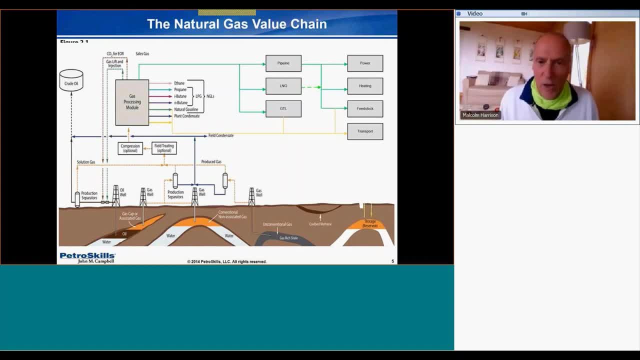 And how do we go about deciding how much we're going to take out in order to maximize the returns that, our dear friend, No one treatment? talk to that. There we go. That's, that's the. that's the. that's the value chain, the oil and gas value chain, actually, rather than natural gas. 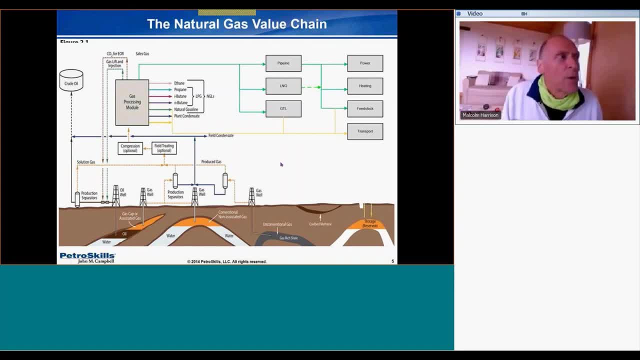 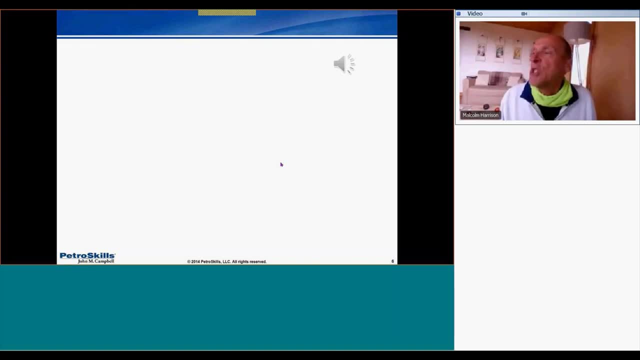 So then we come to another famous philosopher: Um, This, um, this, uh, this. this particular philosopher had the name of Jesse J Um and uh, she came up with a philosophy diametrically opposed to that of Milton Friedman. 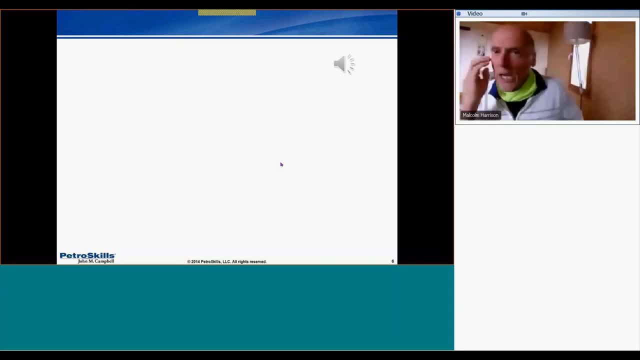 I'm going to try something a little bit adventurous here and see if I can play music over Um WebEx. but this was how Jesse J expanded her particular Philosophy on the purpose of a corporate organization: 321.. Let's see if it works. 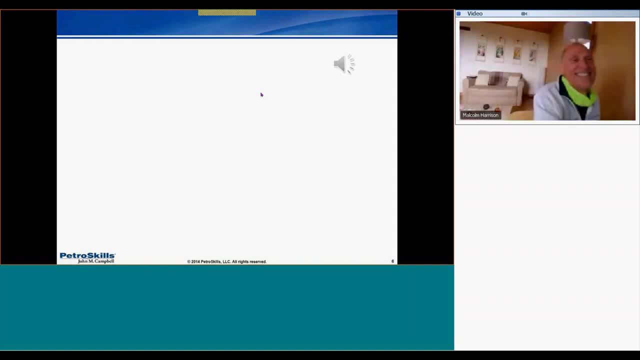 Hey, Oh, Jesse J And Milton Friedman ever met, but I think they would have had an interesting exchange of views becase jesse j. but it was not nothing to do with the money, money, money, money. it was all to make the world dance. um, jesse j was wrong, it's all about the money, money, money. so what i did last week? 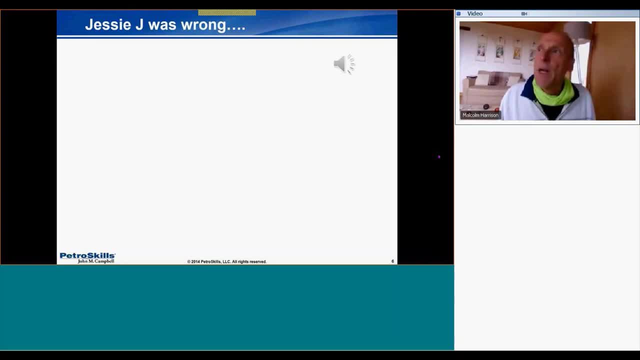 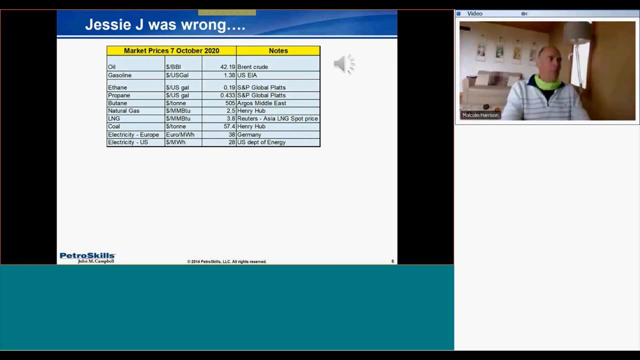 was just go on to the internet and see where the money, money money was last week for the various products that come out of this wonderful oil and gas industry, and you should see those on the screen in front of you. so, as of the 7th of october, oil was selling for 42 dollars a barrel. gasoline. wholesale gasoline prices in the united states were about a dollar forty. you could buy ethane- there's two in the united states- for 19 cents a gallon. you could buy propane for 43 cents a gallon. i i thought i'll wander a little bit from the united states and we'll wander into the the middle east. if you wanted to buy a ton of butane last week in the middle east, it would cost you about 500 back to the us. for a while natural gas in the us was selling at 2.50. 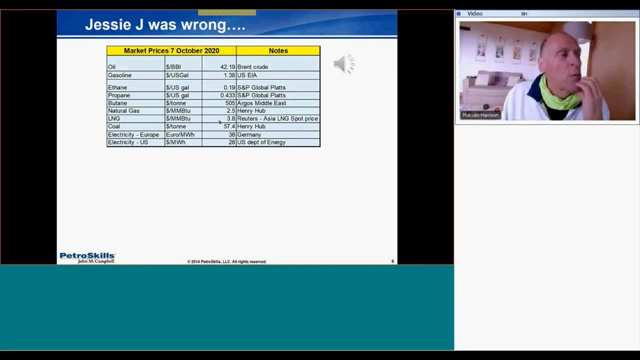 lng. the spot market price for lng last week was 3.80 for each for a million btus. i thought i'd throw coal into the mix as well. not that, uh, but it's a product of the oil and gas industry, but it's uh, um, it's used for generating power. you could. 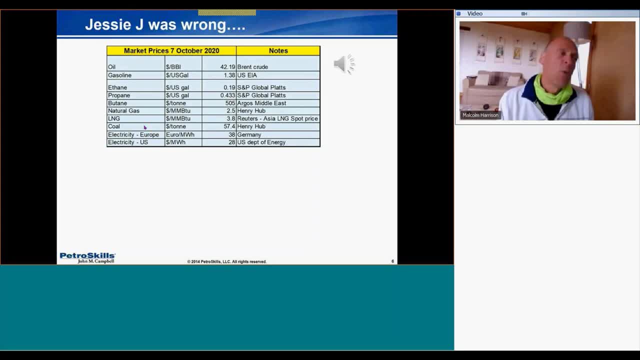 pick up coal for 57 a ton and if you wanted to buy electricity, you can see the prices on the screen in in front of you. about what are we? about? 30 more expensive in europe, um, than in the us. so there you go it, uh, but it isn't all about the money. money, it's about maximizing returns. 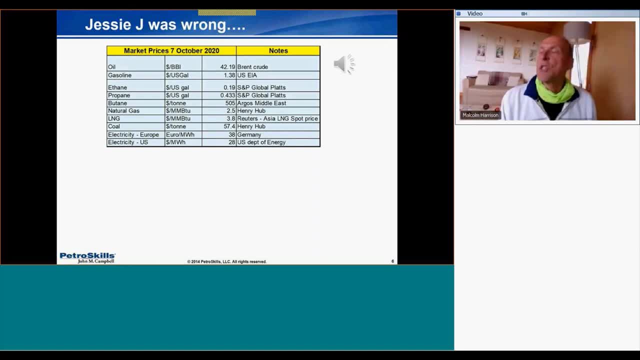 your only challenge is to look at that list of prices and say so, how are we going to operate the facility today in order to maximize returns? um, and and have a crack at one or two questions: should we be maximizing or minimizing ngl production? we have a choice, you see, with some. 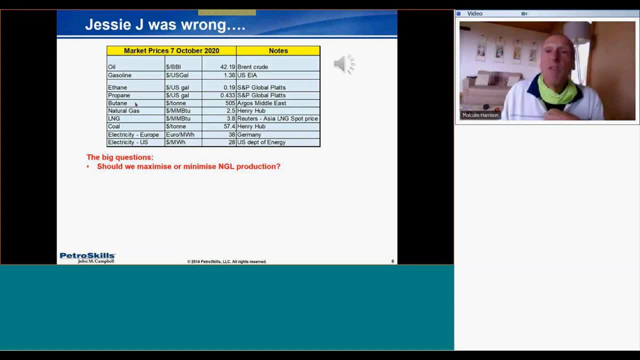 of the um with with um c4s and c5s, we could slip them into ngl production, in which case we could sell them for the price of gasoline, or we could sell them as lpg, which is the best deal. this is. this is a question that you might be able to answer, um. should we be selling gas domestically? 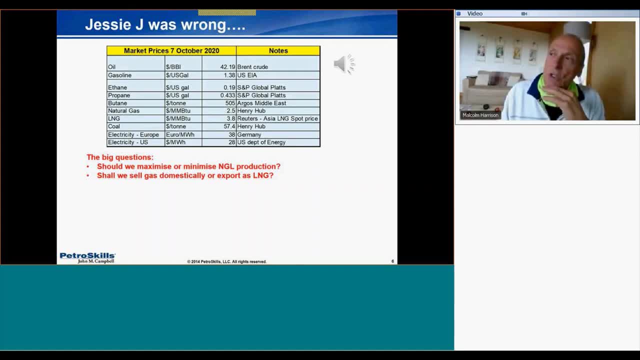 in the us at two and a half dollars a million btus? or should we be liquefying it, putting it in a ship, sending it to asia, re-gasifying it and selling it as lng and making a markup in the us of about fifty percent? 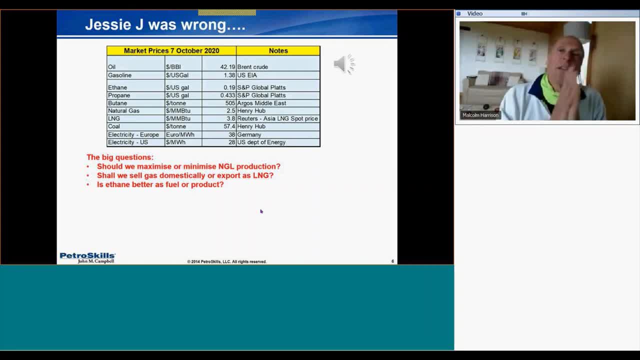 what about ethane? there are options for ethane. uh, we could let ethane slip into the sales gas, in which case we would sell it at two dollars fifty. we could produce it as a separate product feed the petrochemical industry, in which case we'd sell it at 19 cents a gallon. or we could let some of it slip into the propane, in which case we would sell it for 43 cents a gallon and we could take the oil and we'd buy it to an oil refinery and we could let it slip into the oil refineries. how much money is to be made from refinery refining? we buy oil at 42 dollars a. 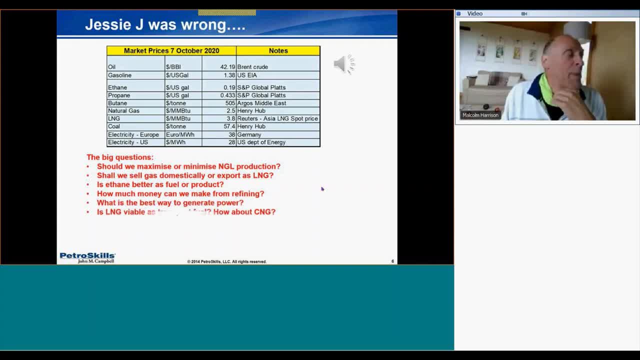 barrel, we turn into gasoline. a dollar forty a gallon, um, and so on and so on. what's what's the best way to generate power? there are choices. is it gas or is it coal? and lots and lots of other questions. the point of putting these up is, um, it's very hard to answer every single one of them based. 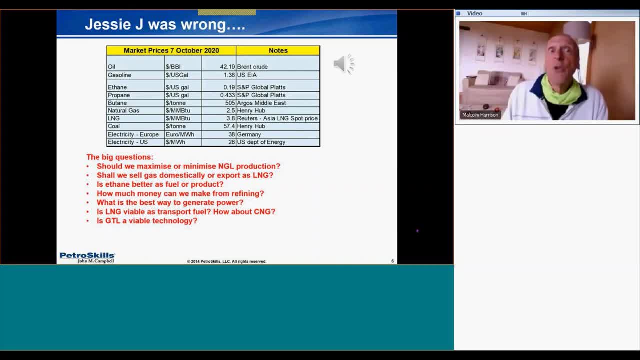 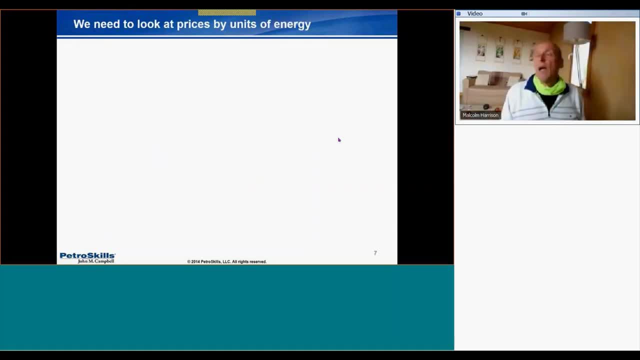 you see before you because of the mixture of units. but if, instead of looking at tons and barrels and us gallons, if you look at the, if you look at those same prices, and there they are again in terms of their uh, the, the cost per unit of energy. 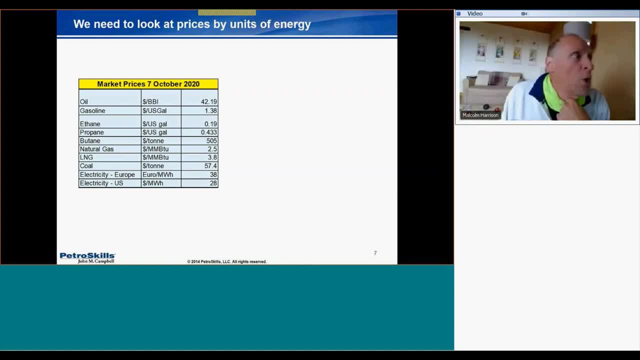 and all of a sudden you can compare them and, of course, when you look at those various destinations of the products, actually, mostly what customers are interested in is buying sources of energy, whether they're measured in gallons or tons or whatever is needed here or there. um, so it's, it's a it's, once you know heating values and densities and various. 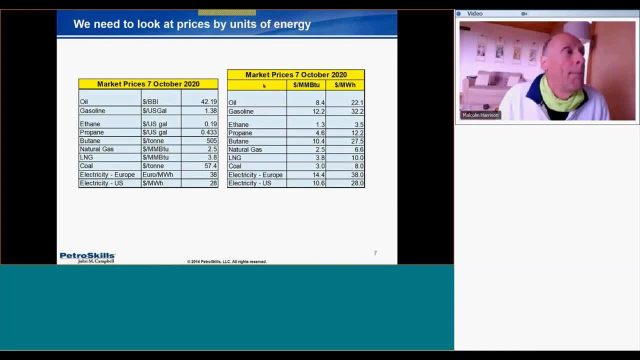 various other physical properties. you can convert them. now you can start to answer some of those questions that i asked before and actually one of the things you, one of the things you notice is: um, we can, i'll, i'll use some btus rather than the. um, the. 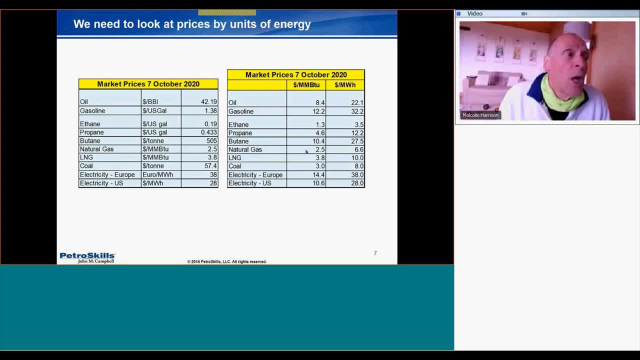 megawatts, the european units. but um, gas was selling at two and a half dollars a million btus oil or gasoline rather, which is what ngls are. we're selling at nearly five times as much. so we should be that first question: should we be trying to maximize ngl production? yes, 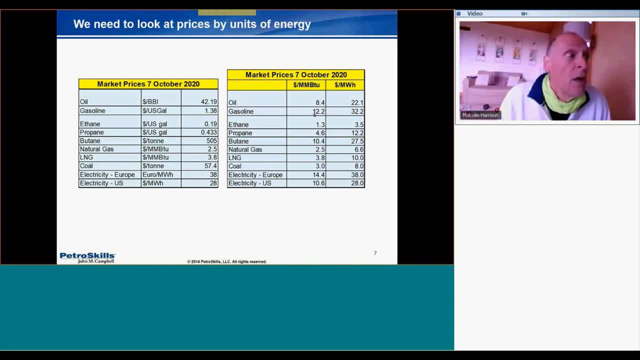 yeah, we should. um, the profits we're making are then made from the liquid products and not from the basis products, and the values are quite a bit, uh, quite significant. take a look at ethan. so these are ethane prices in the us today. it's actually it's cheaper to buy. 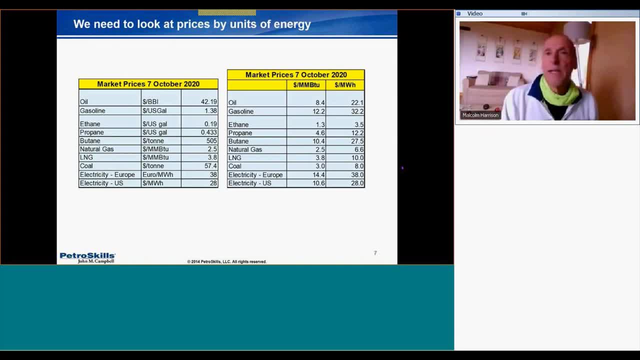 it's actually it's cheaper to buy the income from the us. So what does that tell us about how we should be operating today? I'll tell you what I think it tells us. It tells us if we can slip that ethane Into the, into the propane, and typically you could. you could tolerate 3, 4% of ethane in the propane. 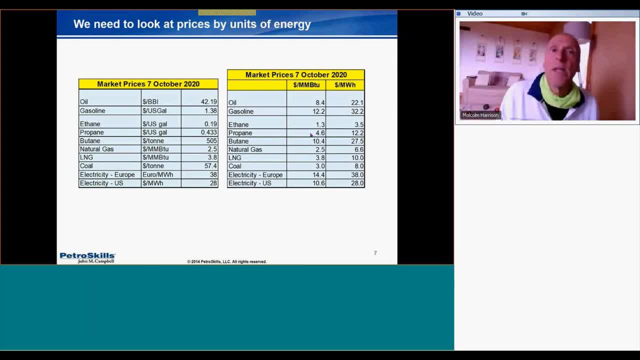 You can sell it for both more than sales class And I buy nearly 4 times the price to get anything. So you should be slipping as much as you can into the propane. You should be slipping as much as you can into the natural gas. 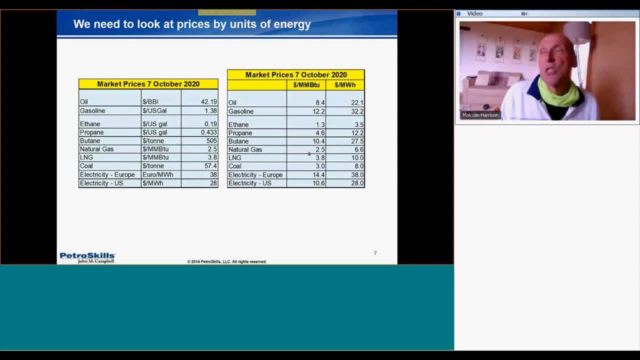 And the 3rd thing you should be doing, if there's any left after that. if you have to take out more in order to meet your product specs, You should be burning it as fuel, because it's cheaper to sell. And the third thing you should be doing if there's any left after that, if you have to take out more in order to meet your product specs, 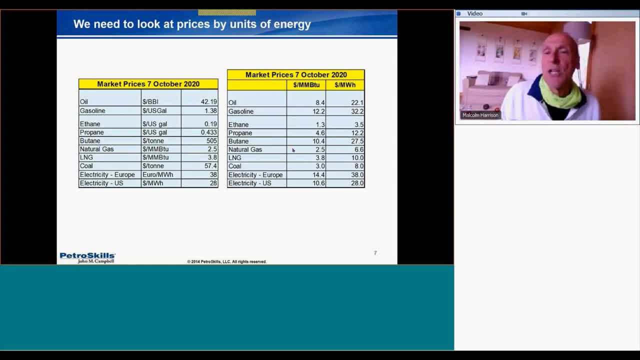 And the third thing you should be doing if there's any left after that, if you have to take out more in order to meet your product specs, It's cheaper to use ethane as fuel than it is to use natural gas and then lose the sales value. 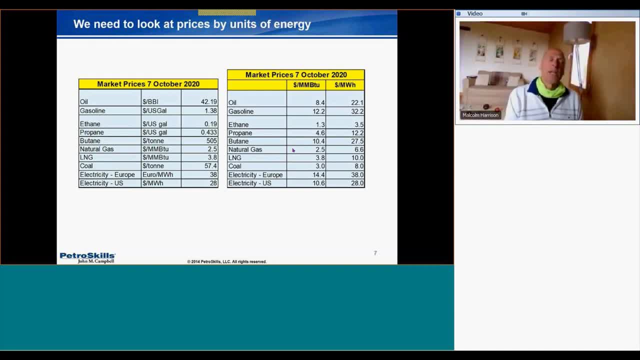 You get the feeling, but there was that question about Should you be selling your natural gas locally or should you be liquefying it and sending it off to Asia. And actually what you see, what you see here, is the margins on LNG at the moment. Are probably amongst the lowest and crashes in economy over the place and also, driven by a surge in suppliers, a number of plants have come on stream. so actually at the moment there isn't much to be gained profit-wise in the world of lng. but if you look back only a year, the energy spot market price was was. two and a half times what it is today. if you look back four or five years, um lng was selling at 18 million btus. but you, when you understand that, you get some idea, if you're ever involved in the in the in in the lng market, why there's such a desperate rush once an lng project has been. 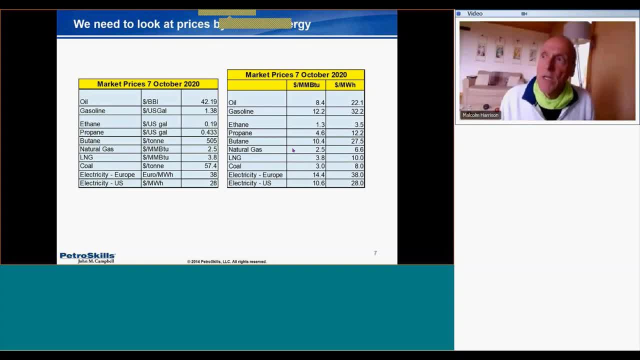 sanctioned to get it to the market and deliver it, because it's the aim, is to it's, to it's the what does the early bird do? does the early bird catch the worm? i think is the uh is the phrase. if you can get to market before the other guys, you can get the premium prices. 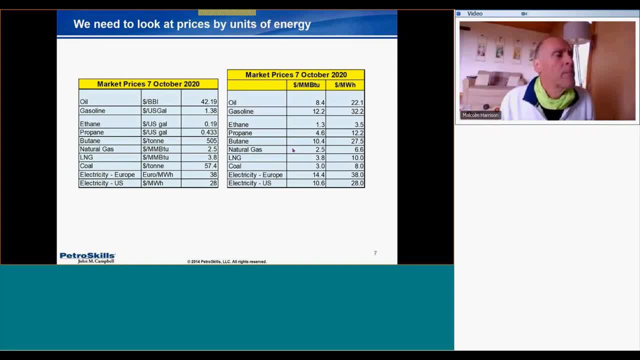 um one. one more thing on that. what about coal? coal's an interesting uh um. should you be generating power with coal or with natural gas? in the us, it's interesting: natural gas wins um, and although there was a push early in the trump presidency to to reinvigorate 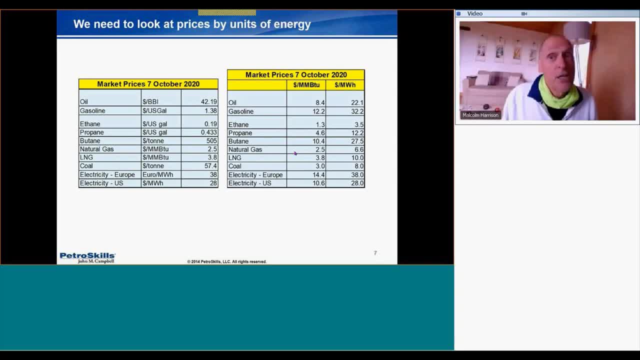 the coal industry. the market would say: actually you're cheaper to run with gas if you hop to europe. we're actually- and i haven't put it on the site- gas prices in europe are about double what they are in the us. it's actually cheaper to generate electricity with coal than visit gas. 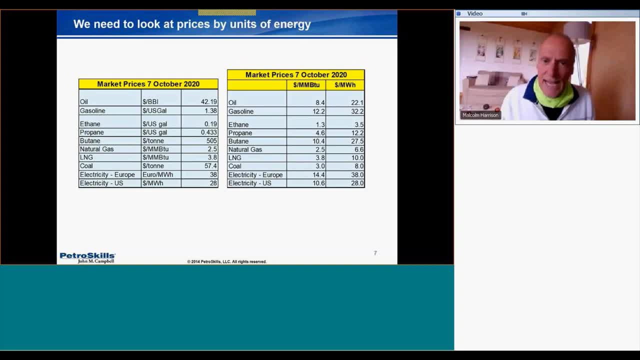 which is why, in the end, the push towards gas for power in europe is driven by legislation, and regulation rather than the, rather than the market. i just wanted to mention two, two more things. um, knowledge of prices does lead you to understand some of the more wacky things. 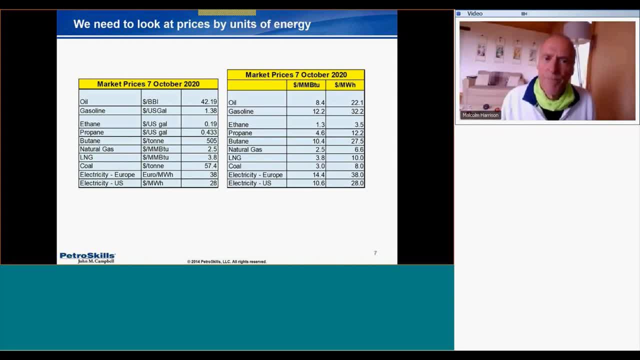 that you see in our industry, some of the uh um hard to understand. there are four refineries in uh nigeria, all of which are shut down, and they're all shut down because the the market for gasoline is government controlled and the price for which the government are prepared to pay for gasoline is less than the price of of oil. 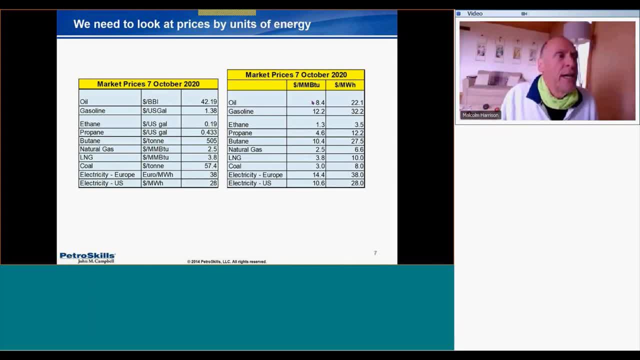 so the the other unusual thing, you see, is that in some instances, companies are are fined for flaring or are not permitted to flare for urban and emergency reasons, and so in some cases there's a, there's an incentive to operate as inefficiently as you possibly can in order to avoid clearing, so that the market and the prices do encourage some. 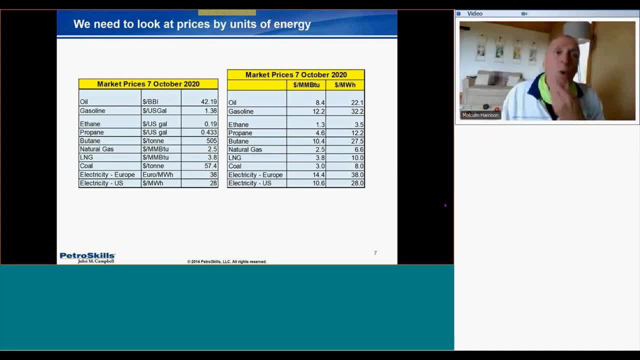 dysfunctional behavior in some, in some cases. but look at that, that was all about day-to-day. that's the day-to-day stuff. so if you were deciding how to operate your facility today, those numbers would give you some guidance as to where which which products are going to give you the best profits. what about if you're not designing? if you're? 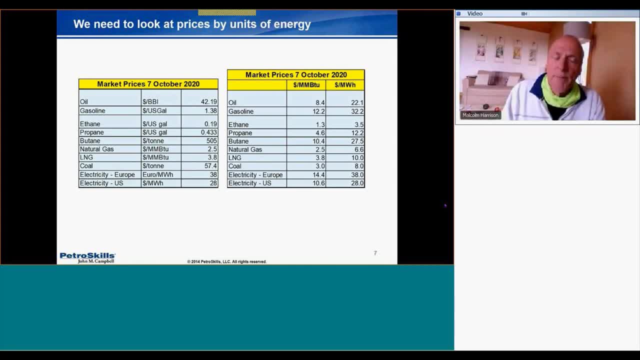 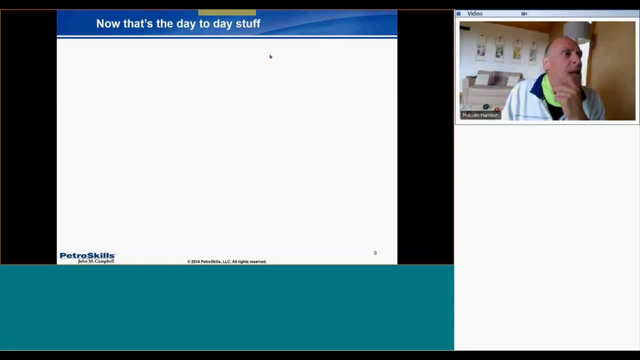 sorry if you're not operating, but you're designing and that is my next slide. i hope you're still all with me. it's quite strange, uh, talking into a talking into a camera and not being able to see the audience. but uh, i'm not going to tell you about these because you're all smart and you remember them. 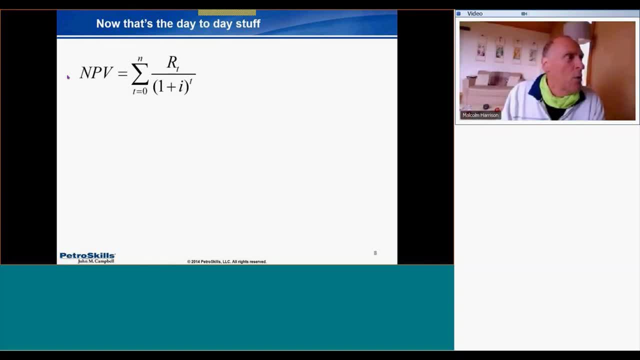 from from from school. but the uh. the net present value of a of a bunch of future cash flows, um, is equal to the sum of the cash flows divided by the, the cost of capital over over time, um. and if your revenue stream is a constant, you've got an equation there. yeah, yeah, i'd, i'd. 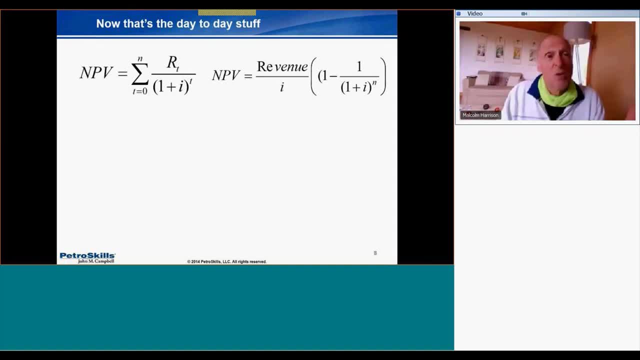 i, i, i would be incapable of deriving these back, but, uh, but, but trust me, they're true, they must be true. i find them on the internet. uh and um. so now, if you look at now, look at um, i'll say market prices, i'll say market prices of the 7th of october, and now we're going to convert. 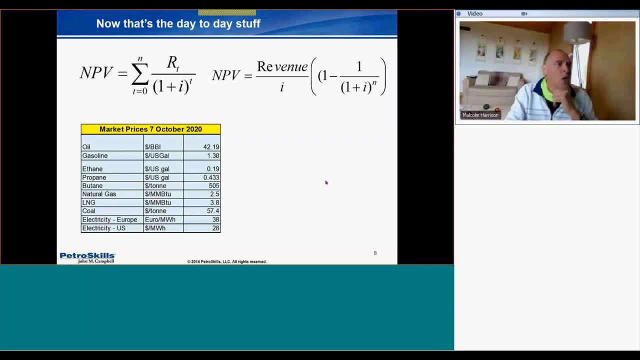 them using mp, the mpd formula, to what is a capital equivalent? a capital equivalent. so what i've done here is is i have assumed a cost of capital of two percent. the cost of capital is is unusually low at the moment. um, and that's where i'm investing for a 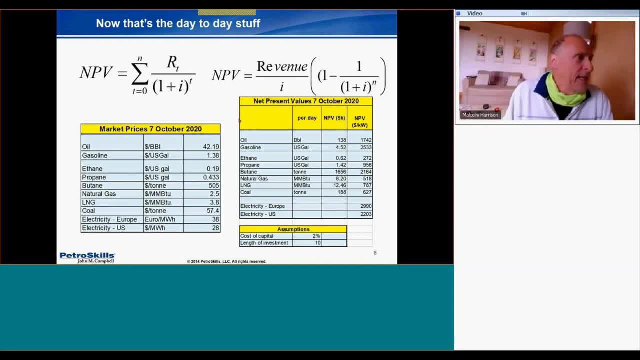 10-year period. and what that tells me is that if i, if i basically plug these numbers into this equation and discount it at two percent over 10 years, um, anything i can do in the design phase to produce product, increased production by an extra barrel a day. as a capital equivalent of 138 000 dollars. so i can afford to invest capital up to about 140 000 for each barrel that i produce, and you'll see. all the other numbers have have been derived in the same way and in the same way that previously i converted to energy equivalents. uh. 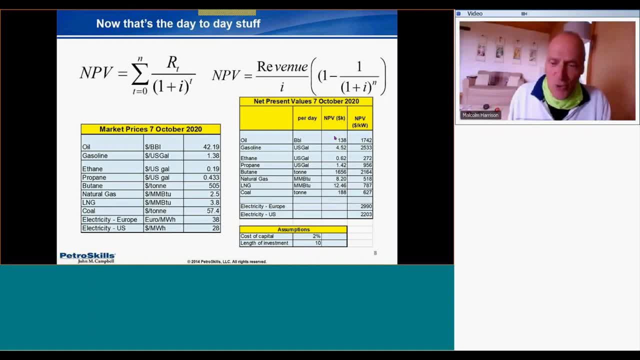 single other prince in the first movie, missing only man富ism. and in the same way that previously i converted to energy equivalents, you have energy equivalent numbers, numbers there. now this is this is this is crude. uh, this is crude and simple. this doesn't take account of of of things like corporation tax and um. 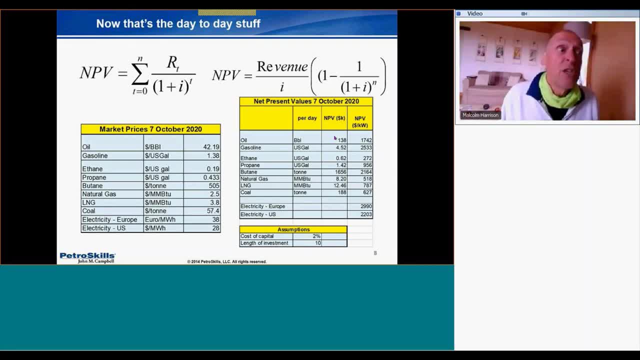 phasing of capital investment and so on and so on. you're in the technical world. this gives you some idea of the commercial benefit of the decisions that you're being asked to take when you put a design together. so now, what i wanted to do was that was to end with some tough questions. i wanted to talk a little bit about the whole renewable. 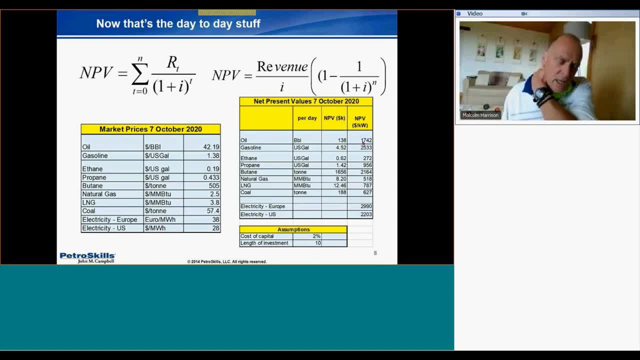 market. you all would have seen that. i'm sure that the statements being made by governments and companies around the world at the moment. shell and and bp have both declared recently that by 2050 that their operations will be carbon neutral. the european union has declared it will be carbon. 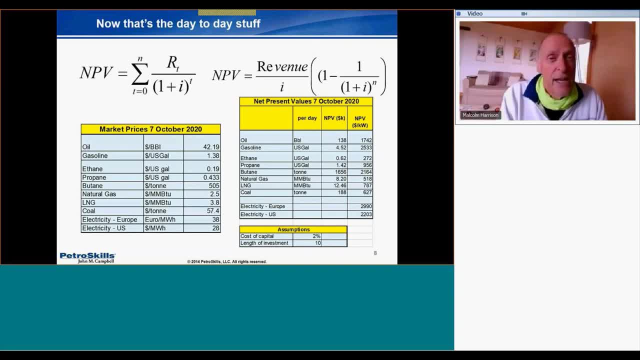 neutral by 2050. china even declared that it will be carbon neutral by 2060.. um, are these things going to happen? hey, i don't know. um, but it does mean there'll be. there'll be changes in our world because they're being driven by major companies and and major governments. 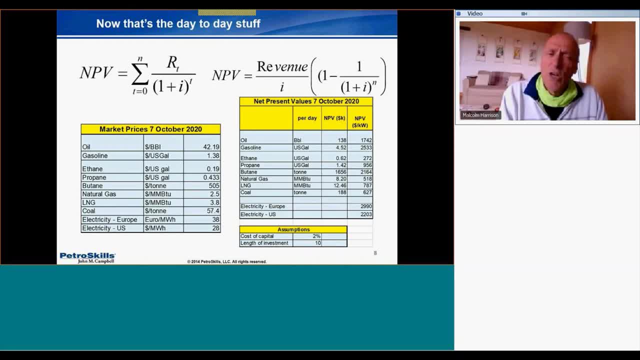 and i guess the question, the questions i wanted to have a go at was so is- is: um, just how far away is solar power from displacing gas or coal? um, what about wind? just what is going on in the transport industry, i mean, um, it could be about 100 million cars a year, or a billion cars a year. 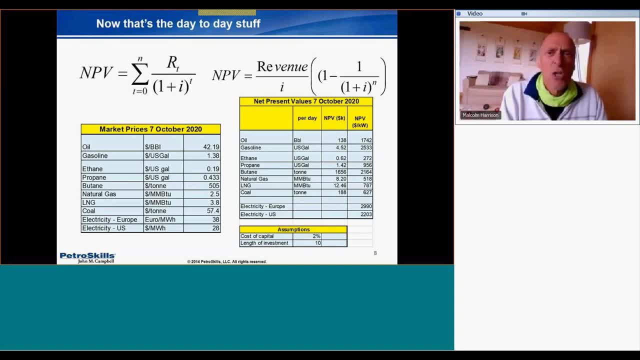 um or others that could be. well, that could be a huge market capitalization. um, you know the, the, uh. the other thing that's important to note: um, which is like you've got, um, you've got companies like uh or a company like tesla, um, that's got a market. 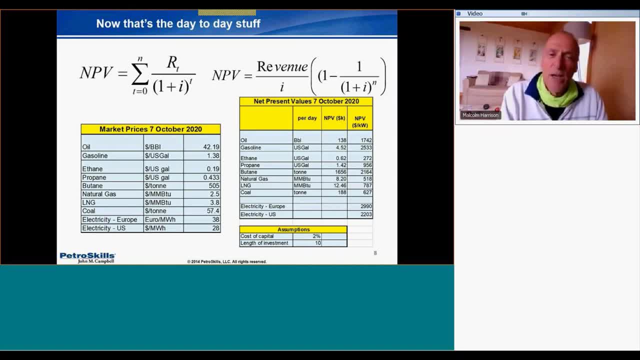 capitalization that's that is greater than exxon, exxonmovil um actually tesla um. tesla produced 350 000. There's other questions as well about how you value once you've got these numbers, how you value companies. Saudi Aramco has enough oil in the ground to produce at current rates for another 100. 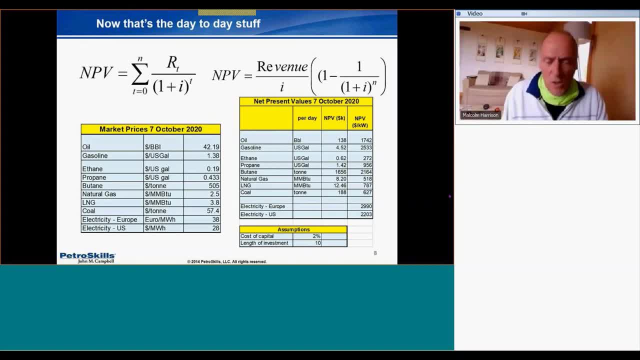 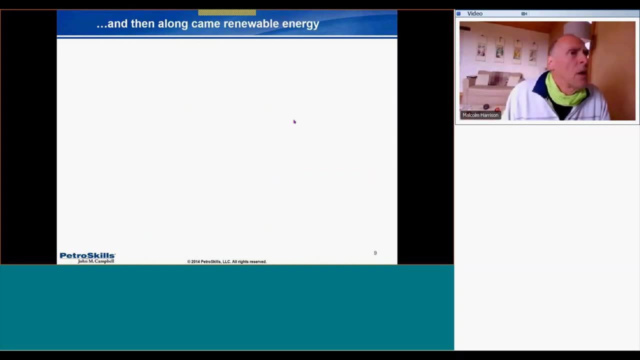 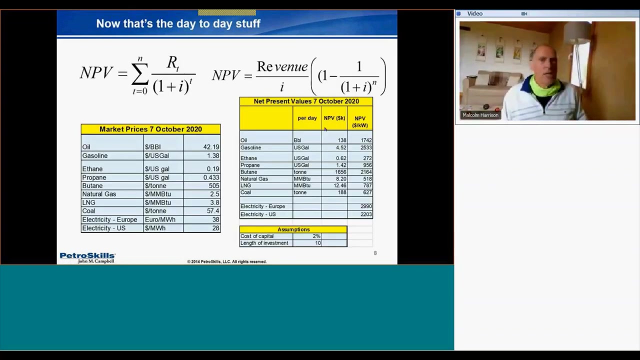 years. But as the world is weaning itself of oil, how do you value those assets? How do you value Saudi Aramco? There's a couple of numbers on this screen that I'd ask you to remember. The first is electricity in Europe. The capital equivalent of a kilowatt of energy in Europe is about $3,000.. Right, $3,000.. If I spend $3,000 to generate a kilowatt over a 10-year period at a 2% cost of power. 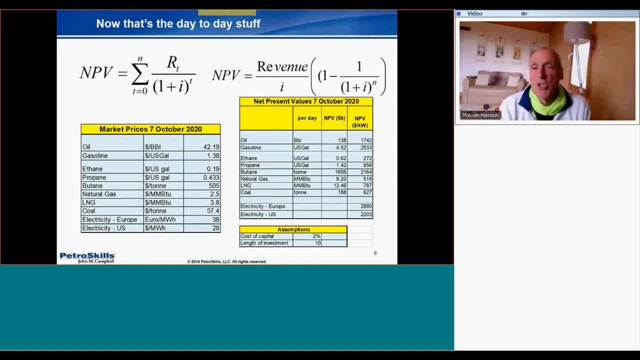 then I'm just about breaking even. The capital equivalent of a gallon of gasoline is about $2,500 per kilowatt. Just remember those two numbers: $3,000 for power, $2,500 for gasoline. And then let's look at it. 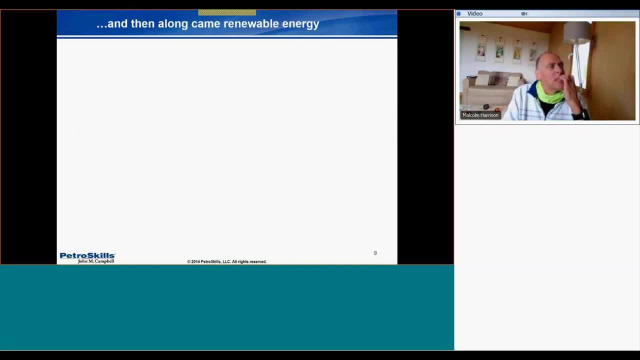 And then along came renewable energy. This is taken from a report from the International Renewable Energy Association. It was published in 2019, so it's a little bit out of date, but not too much, And it shows the falling cost of solar-generated power over a period of about 10 years. 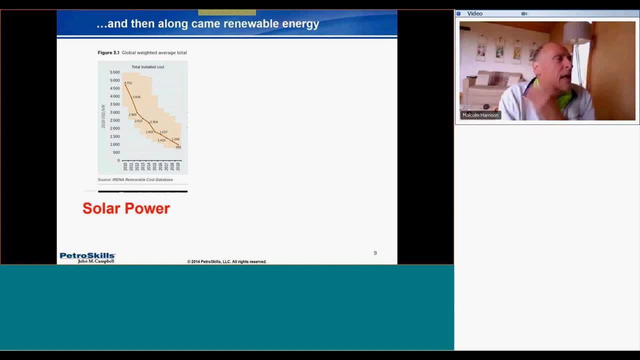 And solar panels are capable of delivering power at a cost of about $1,000 per kilowatt. Remember our base number was 3,000.. So solar power is something attractive, isn't it? Onshore wind can generate power at about half the capital equivalent of current wholesale power. 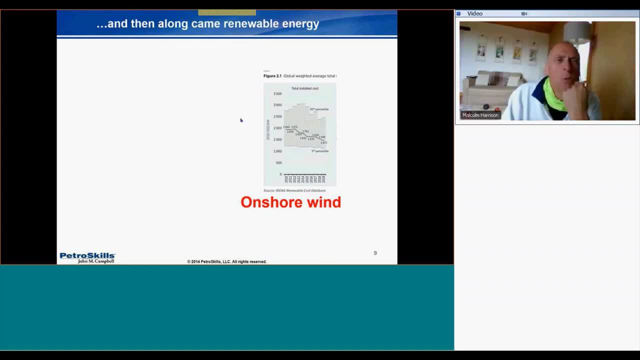 Current wholesale prices within Europe. So onshore wind is somethingly attractive, isn't it? Offshore wind- if it's 2019, is arguably just about competitive. Now, of course, if you didn't all have your microphones muted, you would be screaming at me now, wouldn't you? 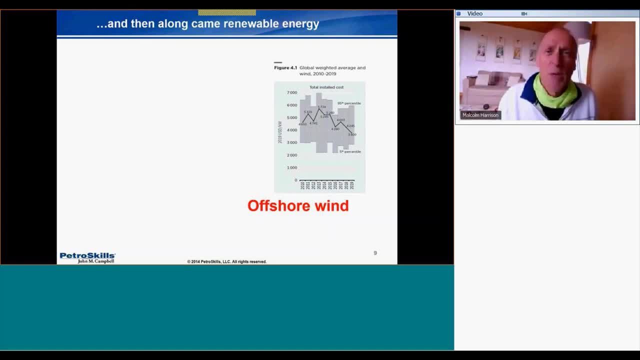 You'd say you're an idiot, You've forgotten something. Thank you, And I have, And I have. And there are very good reasons why the last three statements I made are not true. There are very good reasons why solar, onshore wind and offshore wind are quite a long way from being competitive with hydrocarbons at the moment. 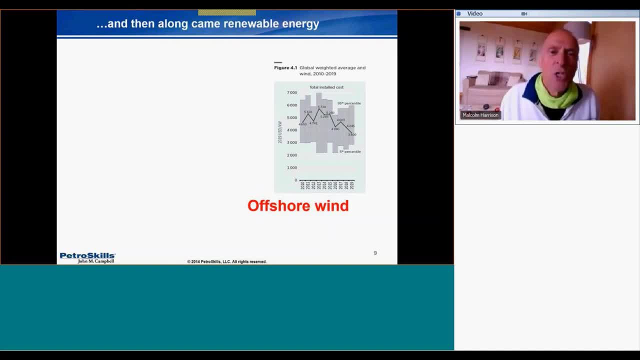 If you want to come back for part two of the lecture, part two of this series, we'll talk about why that is. The other one that I wanted to leave you with Was batteries. Do you remember the number that we took away for gasoline? 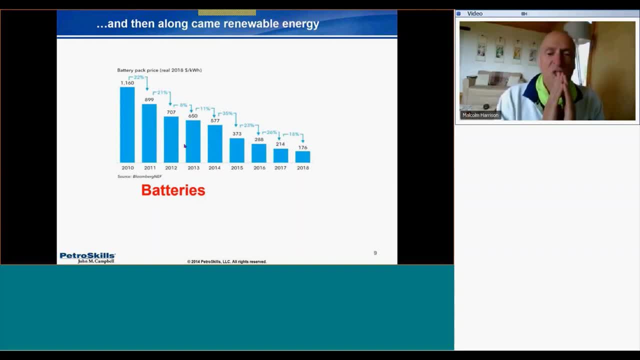 The capital equivalent of a gallon of gasoline was about $2,500 for every kilowatt. I can buy a battery pack for about 10% of that, So clearly batteries are also somethingly competitive, aren't they? And of course the answer is no, they're not. 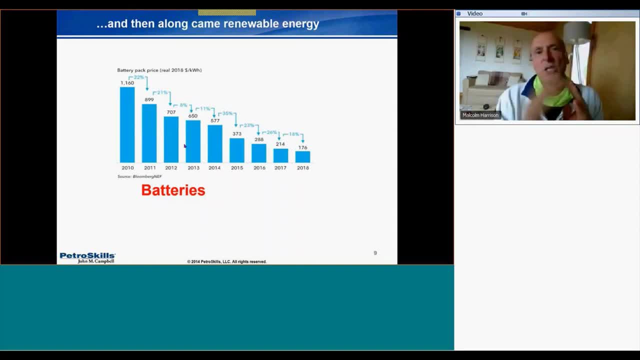 And the secret as to why, And the secret as to why they're not, is contained in part two of the series. Of course, if you've already worked out the answer, you don't need to come along to part two. That is all I wanted to say today, ladies and gentlemen. 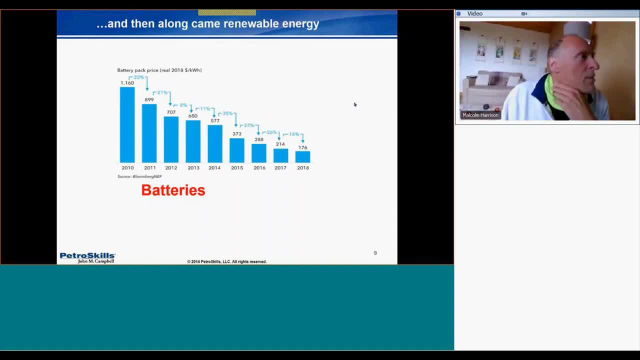 I am getting regular requests on my screen for annotation. I'm quite sure what that means. So what do you take away from today? It's only really. I'm only trying to leave maybe four or five messages. The first is when we think about prices, think energy and not tons or gallons or millions standard cubic feet. 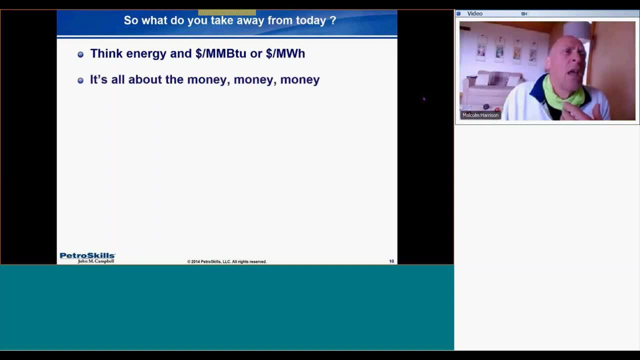 Think energy. Remember, it's all about money, money, money. Remember Jessie J. Do not follow the philosophy of Jessie J, She wasn't as smart as Milton Friedman, But it is all about the money, money, money, money. 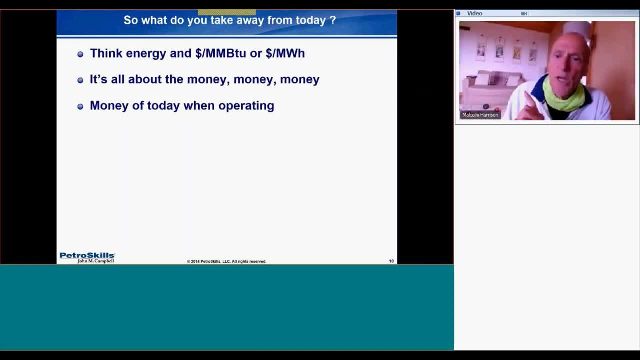 But it's about money of today when you're operating, market prices of today when you're operating, And it's about money of tomorrow- capital equivalent and MPVs when you're designing. So what we've done today is we've taken step one. 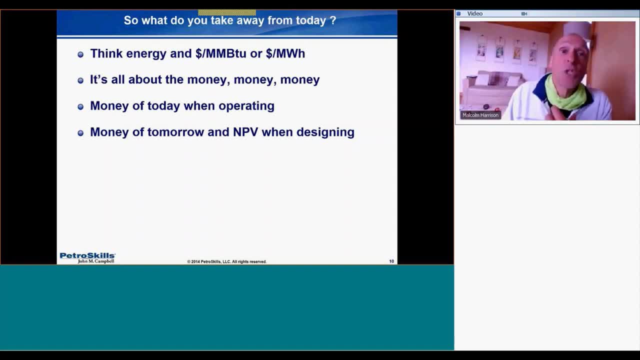 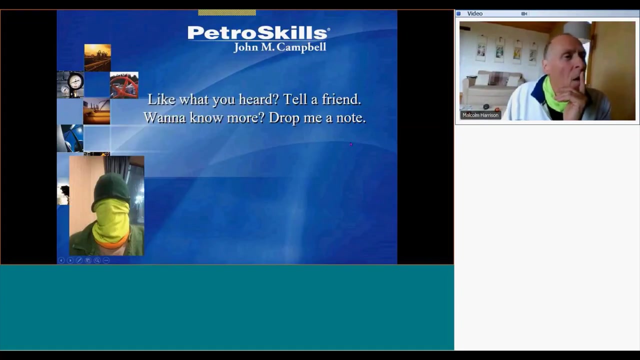 Step one on a journey of five steps. five steps which are all about understanding how to find the money: money, money. Ladies and gentlemen, I will leave you there And I just make a couple of requests, If I could. 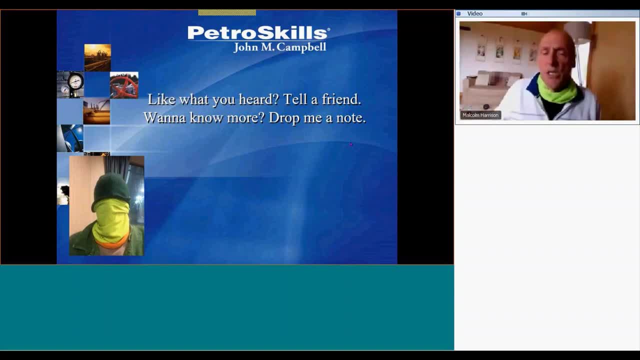 Exposing. If you like what you heard and you're all still on the line, can you do me a favor and tell a friend? tell a friend. if you didn't like it, then keep it to yourself. If you want to know more, if you are interested in step two and step three and four and five, then drop me a note or drop a clear note. 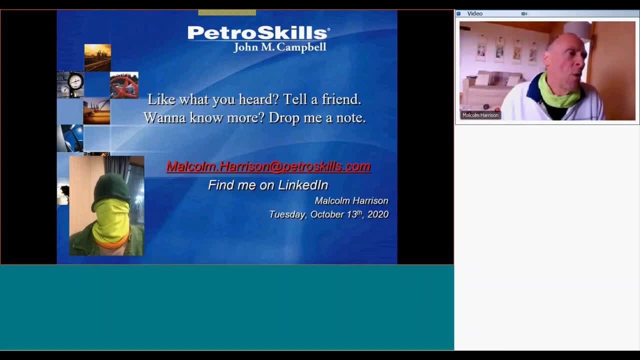 That's my details on the screen in front of you. Petroskills email address: You'll find an easy to find on LinkedIn. I'm not going to play. Maybe at the end of this we'll ask for feedback forms or whatever. 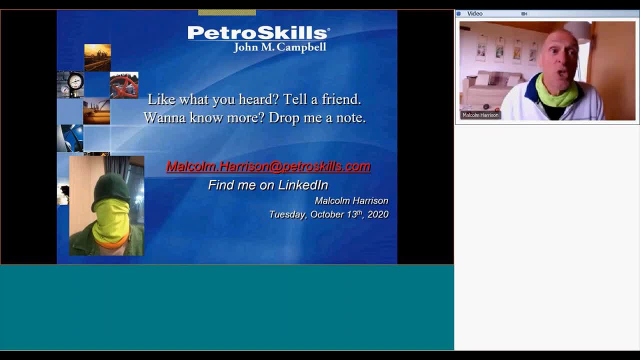 It's not something that I'm asked for, but I do appreciate positive comments. insults, abuse- Anything is helpful if, at the end of this, You have any thoughts that you'd like to share. So that's all I wanted to say for now. 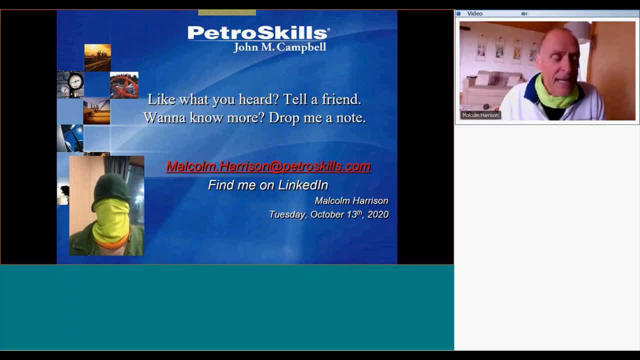 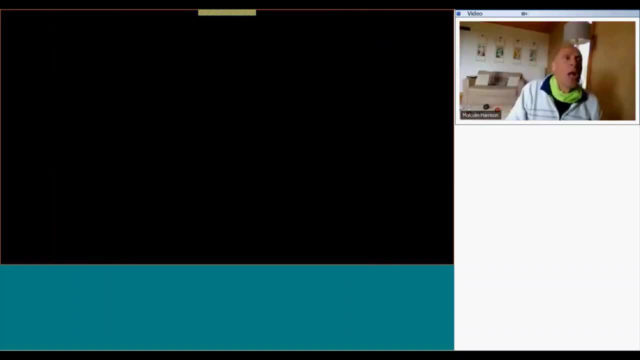 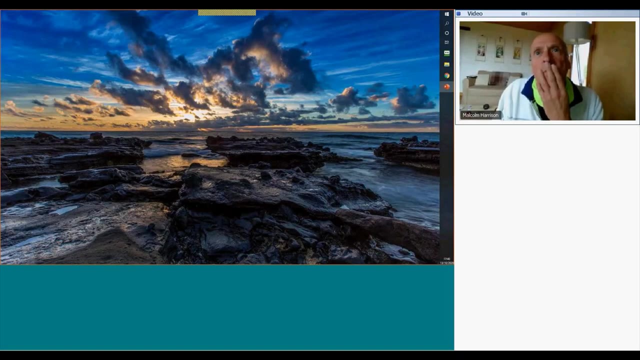 And I think that means That I hand back to clay and clay is going to ask me lots of embarrassing questions that I'm not able to answer. Yeah, thank you, Malcolm. So yes, I do have some questions here and we should have some time for a few more, So continue to put those in the chat. 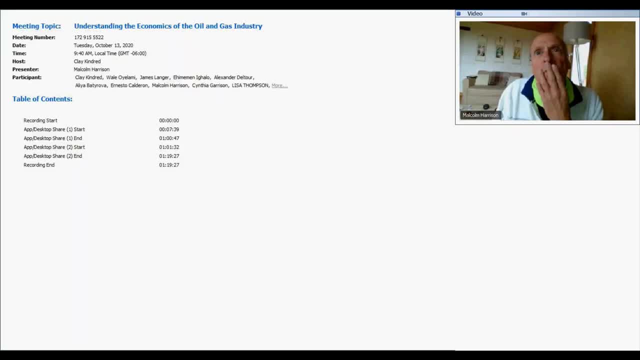 If you have them, and real quick, before I get to those questions. as Malcolm said, This is part one, And so, in addition to sending out the recording of this section, I will certainly send invitations to the next one that we schedule. So to jump to our first question here, this was from the natural gas value chain slide where you went over there. 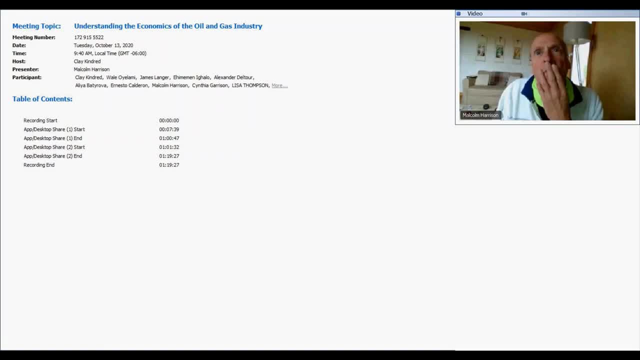 The question asks: what are some examples of feedstock? Some examples of feedstock? That's a nice open question, Can I? can I put the slide back up? Sure, Sure, Yeah, You're still presenter there, I am, Let me. 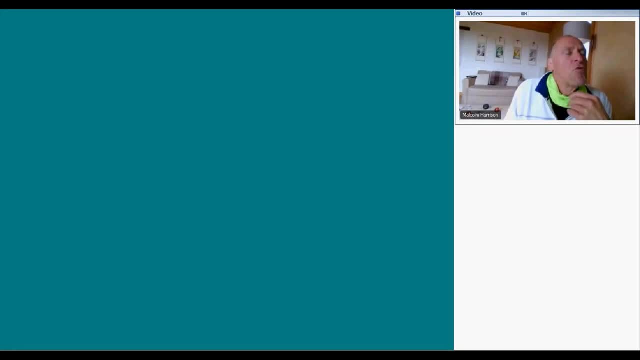 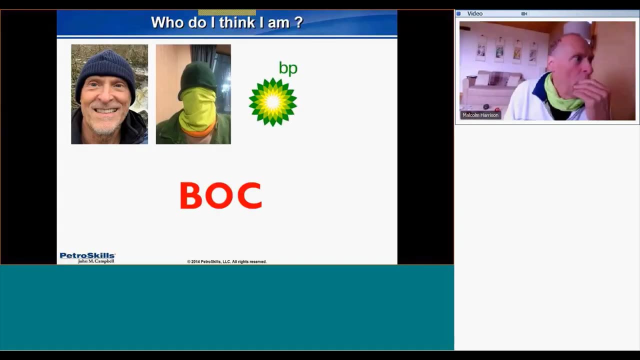 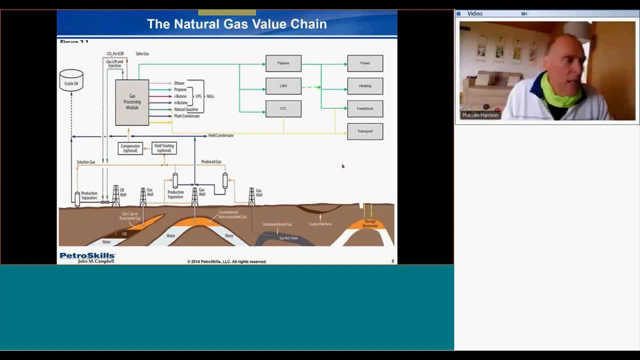 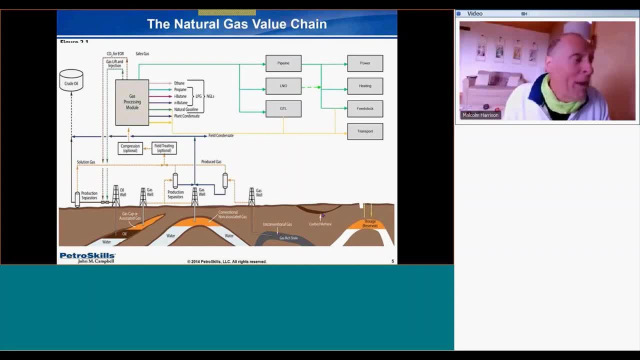 fields which are pretty much entirely gas- Shell gas, I think, coal bed methane we've got here- which is essentially no liquid products- through to, on the other hand, really really heavy oil fields. Now the way in which you exploit those varies enormously and their value varies enormously. 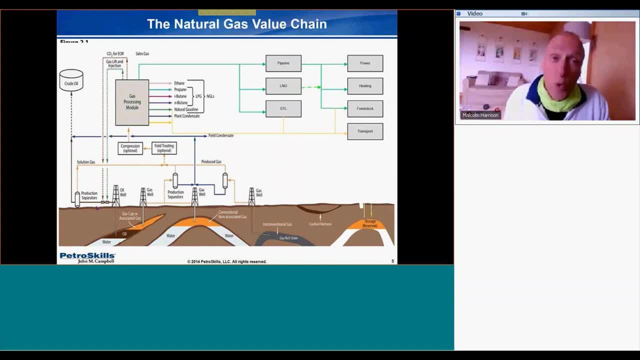 I don't know if I'm in any way answering the question. The important takeaway that I think, though, in terms of feedstock, is: just remember the money. the money is in the oil and is in the gasoline and liquid products, and not so much the gas. 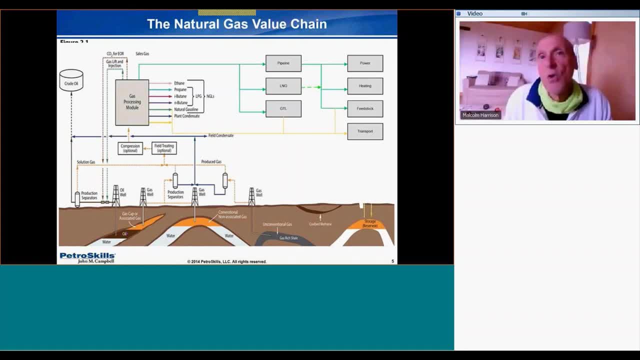 So typically the heavier the field is in oil and condensate, the more long term value it's got, And of course, with the disadvantages. I don't know if I addressed the question. if the person who asked it has got some means of telling me, then I'd be grateful. 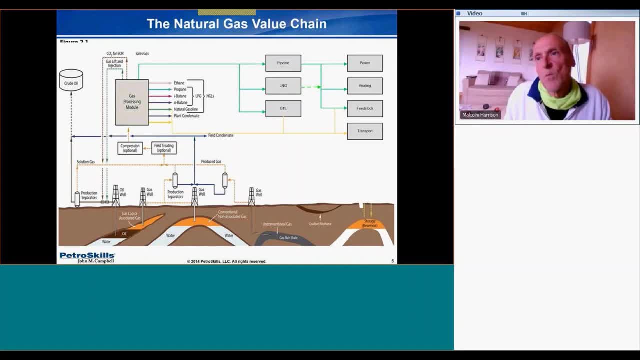 All right. Next question is: What are the parameters- the economical parameters- that need to be considered while deciding grassroot refinery configuration? Oh wow, I need to know the name of the person who asked that. Can you repeat the question one more time, please? 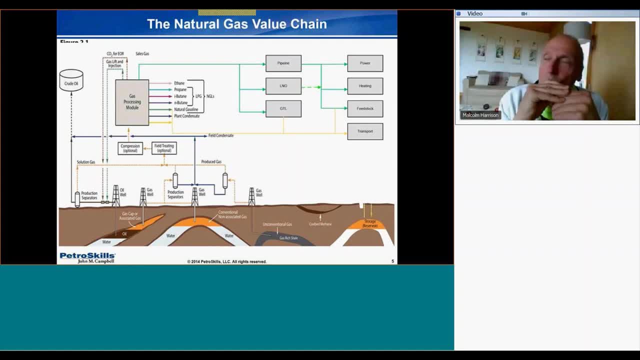 It says: what are the economical parameters that need to be considered while deciding grassroot refinery configuration? The economic parameters: grassroot refinery configuration. wow, that's tough. wow, that's tough. Well, top of the head start, I wonder who's thinking about a grassroot refinery configuration. 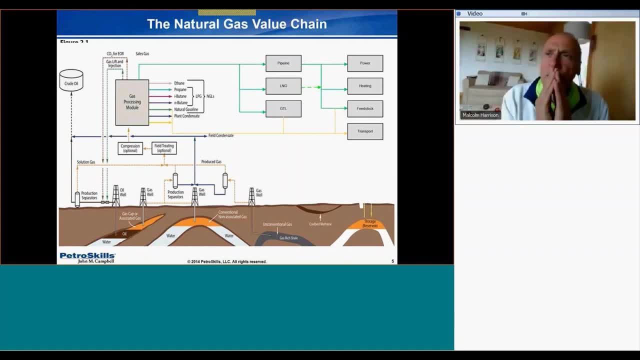 at the moment, Because what's going on in the industry? it's hard to see. there's going to be a need for much refining capacity. But scream at me and tell me I'm wrong, I'm wrong, I'm wrong, I'm right. 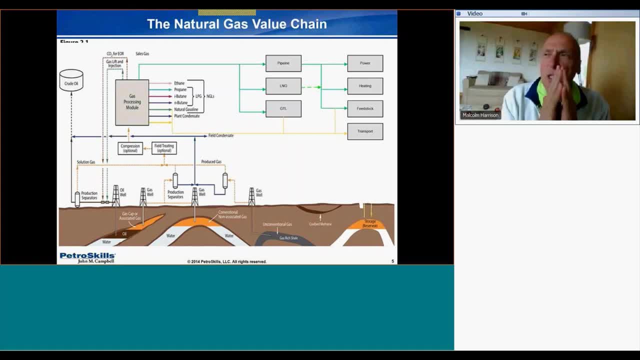 I'm wrong in your view, I guess then it would come. if there is, then it's going to be driven by some strategic or political or domestic purpose, but the economic, the economic parameters, it they'll be, they'll be driven, they'll be driven by. 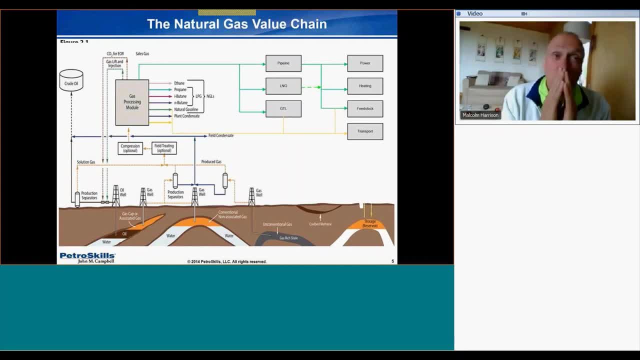 the previous question, the different, different oils, different compositions, different values, but those are mostly reflected in the and the prices in which you you buy them. and then, secondly, it will be driven by, to an extent, local market, um, and some of the prices that we talked about just now i mentioned. 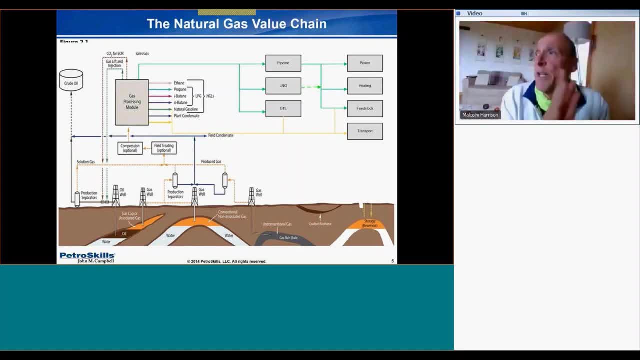 you know, nigeria, where no one, nobody's going to build a grassroots refinery in nigeria because uh the the market is, is is controlled and uh gasoline is given away. but i guess that the economic parameters are going to be essentially what you perceive as being the long-term value of the. 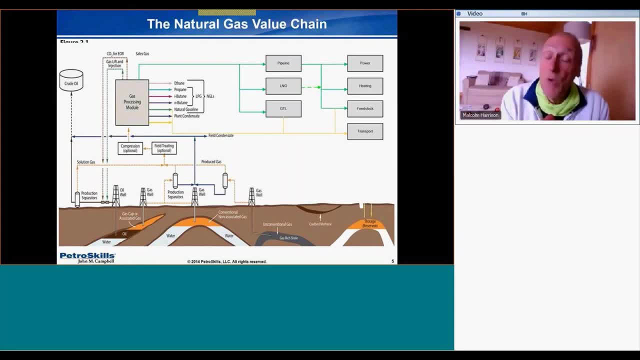 different components, um, you know, starting with with lpgs and gasoline, the values of which we've talked about, but then going through um, napfers, um, which will need a local market, probably to be to use it as a petrochemical feedstock, the heavier fuel oils that are used for transport, and so on. i'm just 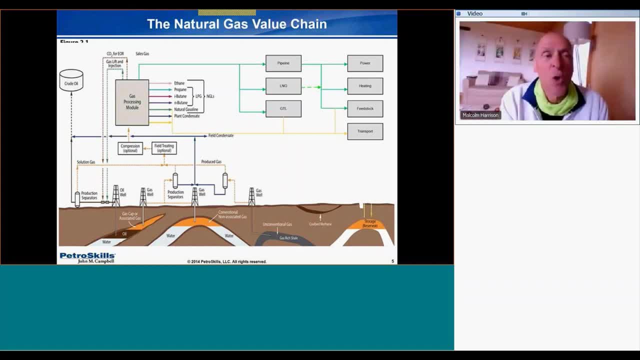 i'm just rambling at the moment. the best thing i could probably do is to stop, because the question is a little bit too hard for me. fair enough, okay, uh. next question. this one says we see hydrogen discussions a lot and have not touched about it in this session. 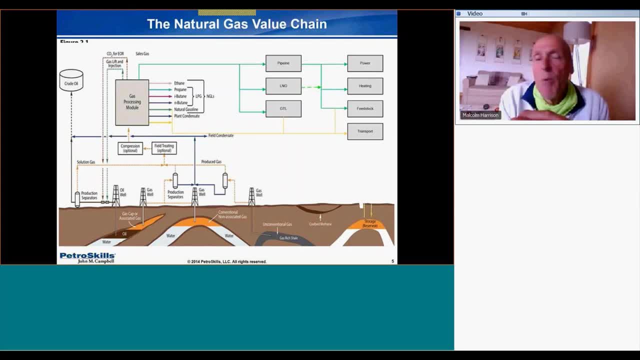 can you explain about hydrogen position in the fuel chain? uh yeah, i'm wondering if i'm going to live long enough to see the hydrogen economy. obviously that's the um, the picture for the future, um, and the future not being not being that far away, um, carbon neutral by 2050, 2060 or whatever. 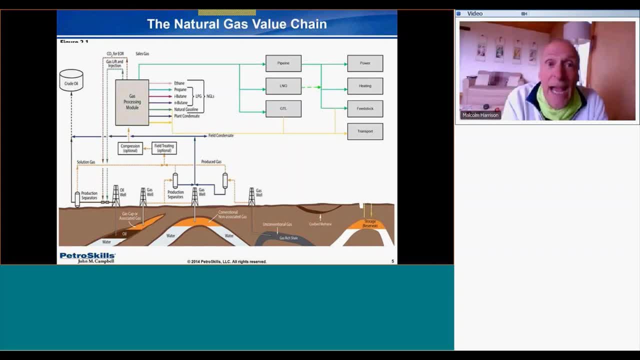 is that hydrogen will will replace natural gas in many of the current uses. it has the potential to be a transport fuel um. there's enormous pipeline infrastructure in um in large parts of the world so it can be easily easily transported um the issue and maybe, maybe it will. 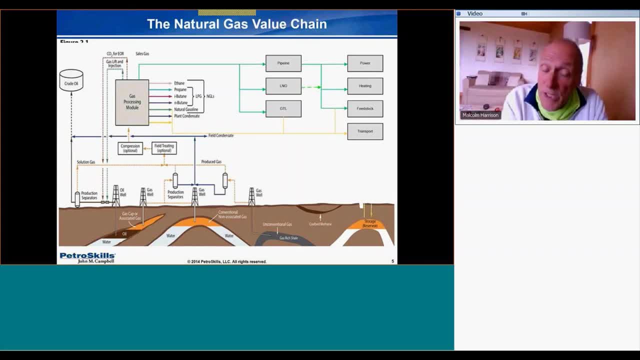 get there? the issue, of course, at the moment, where, at the moment, is, although the technologies are there in order to just save the environment, will it be be? it's a big and very expensive problem. it's more expensive than um on its own and, of course, the the main, the main. 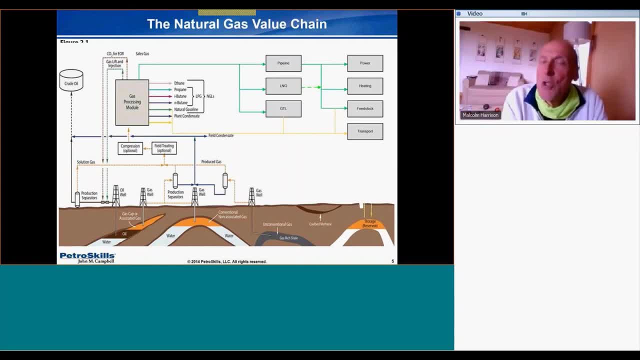 source at the moment of um, hydrogen um- is by cracking a hydrocarbon feed source, um, so you're not actually taking co2 out of the um, out of the production train, unless you can sequester it and stick it back on the ground. If I was able to predict the future, then I would be much richer than I actually am. 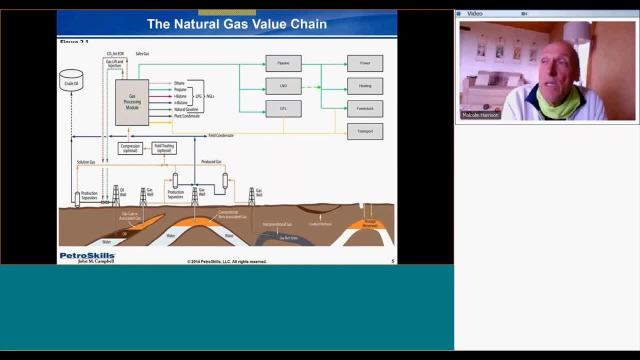 But the technology is there. You can see that there's the possibility of green hydrogen, which would be hydrogen generated through renewable sources, vegetation or whatever. But something significant has to happen on the technology side before it's viable, Or what actually seems to be now almost inevitable. something significant has to happen on the 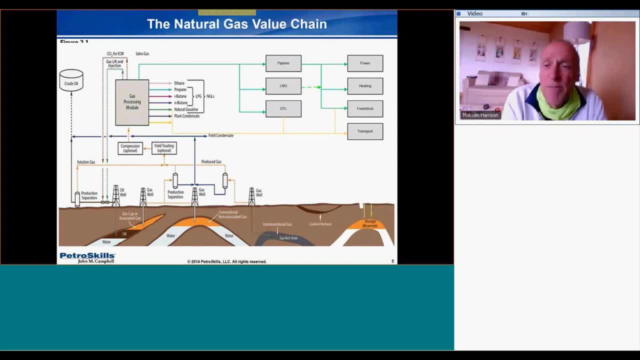 regulation side, such as significant carbon emission pricing or something like that, before it has a place. I don't think the challenges are predominantly technical. there are technical opportunities, but in the end it's going to have to be pushed through with legislation, I'm guessing. 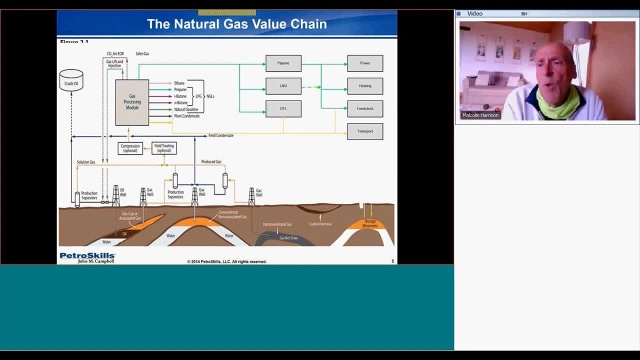 In a way, I'm flattered that people would ask me questions that are this complicated. These would be more suited to somebody on the United Nations Council or maybe the International Energy Agency. Okay, Next we've got a comment and then a question that are somewhat related. 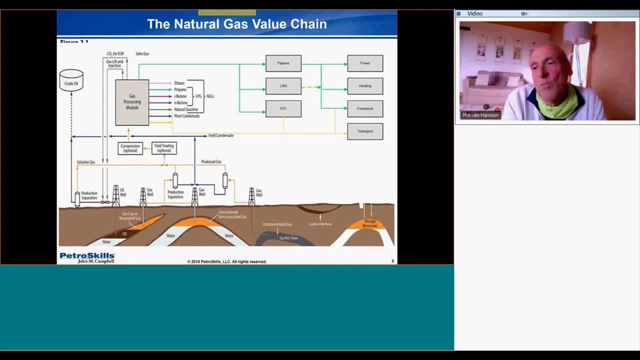 So the comment was that subsidized market prices, Okay, Are not necessarily a fair comparison. And then a related question from someone else asking: does the solar cost per kilowatt hour include tax breaks? Yeah, very, yeah, I think I can answer that one. 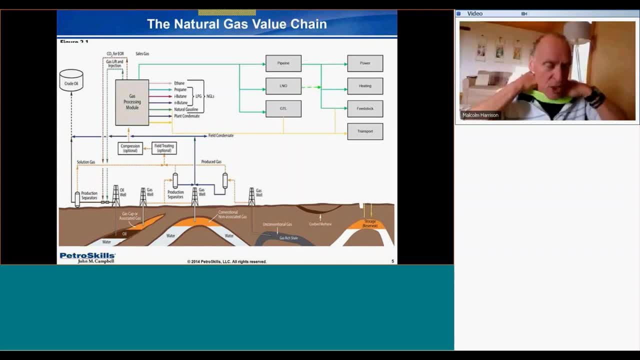 And the answer is no. The answer is no. The numbers as they were presented are capital costs against the power of the solar, The power that a solar panel will produce. I did I missed two bits that if you come back again I'll tell you about. So it's not nearly so attractive as it appears in the way that I've presented it. I have to agree with the first thing: it isn't a fair comparison to compare subsidized market prices with markets that are not subsidized, But of course that's precisely what we're talking about. 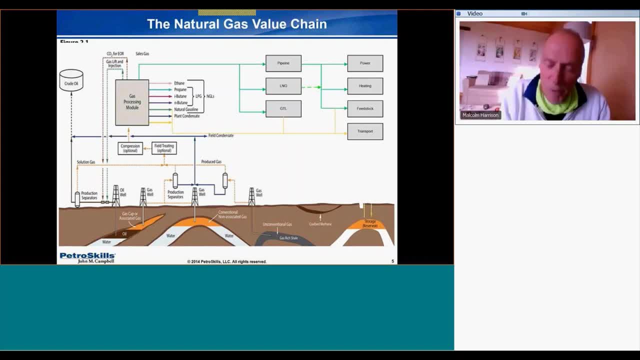 Okay, That's exactly what is going to happen if people are really serious about reducing carbon emissions, because it's only going to happen by markets being subsidized or those that are not currently subsidized- ours, the oil and gas market- being penalized through carbon. 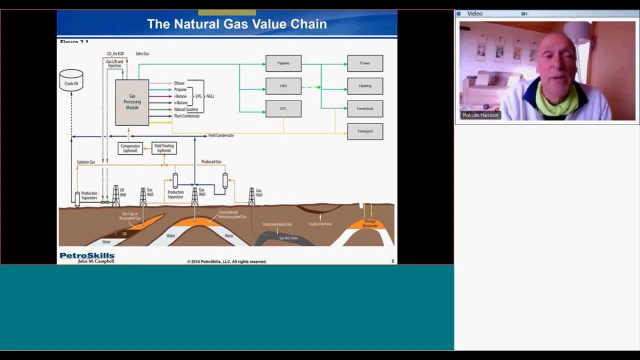 taxes and just regulation that prohibits certain activities. So it's right to say that a strictly Okay Technical engineering level. it's not a fair comparison. But a big player in the energy market in the future is what will be will be governments. 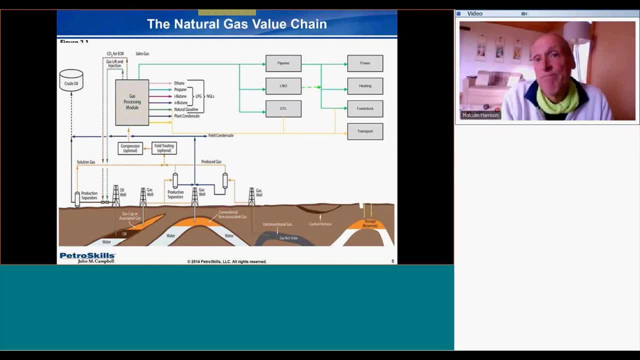 and legislation and they'll, they will drive that, Can I just just so I can avoid asking any more questions. could I ask one question back to the audience? I just, I see there's still about 120 people who are on the line. 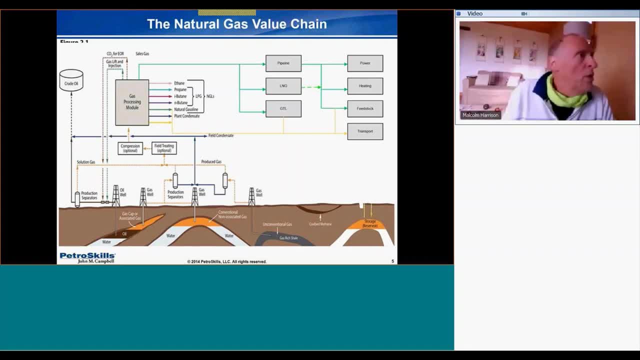 If you, if you, if you look Okay On the, the top of the, the, the, the WebEx menu bar at the top, I think if you click on the participants box, but somewhere in there you'll see the facility to, to, to. 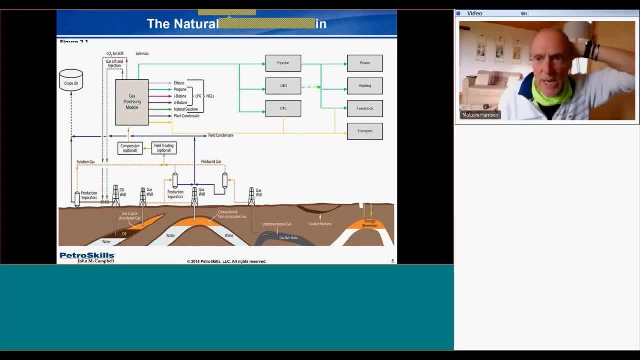 to vote. There's on my screen here there's a little green arrow and there's a little red arrow And I'd just be interested. I wanted to ask two questions. The first is Okay And I said: please be, please feel, feel free to be to be harsh of of those who are still. 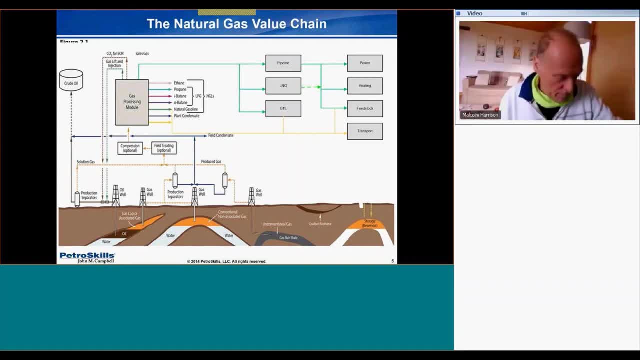 on the line How many people got any benefit from the last hour of their lives. If you've got a benefit, could you click the green tick, And if you didn't, could you click the red cross And we'll see if this works. 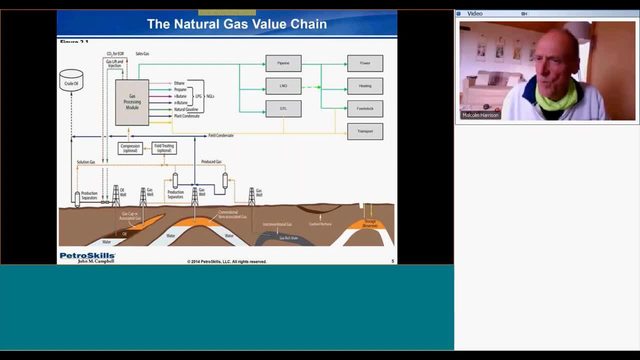 Okay, Okay, All right. Lots of green, Lots of green checks here, That's good, Yes. And lots of lots of people slowly finding out where they, where the green and the red buttons are. That's good, I realized. actually, in asking that question, I took a serious risk of ruining my evening. 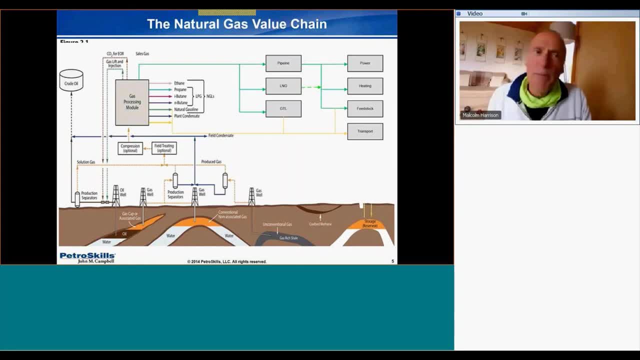 So, thank you, That's resoundingly positive. Okay, And how many people would be interested in part two of the series, which is which is talking a little bit more about? oh, Clay, I might need your guidance on how to clear. 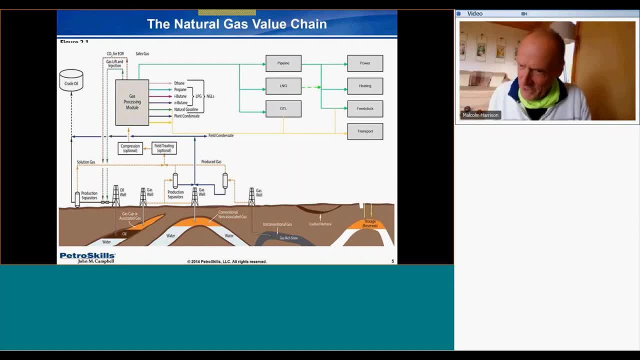 those these results and go on to the next question. You know how to do that. Yeah, If. if you clicked either yes or no, if you just click it again, then it will remove it, Right, That's great. So I'll wait for it all to go back to zero. 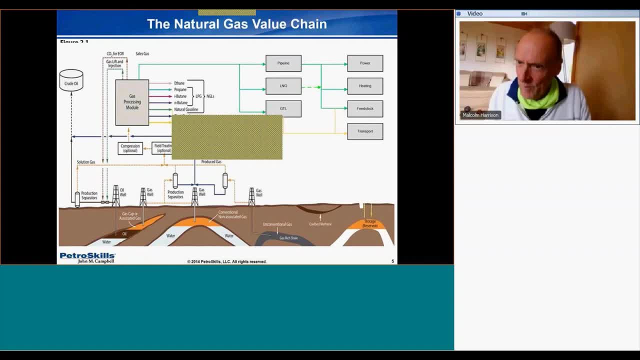 I got that. That was resounding positive, So thank you very much for that. It means that I I didn't, I didn't waste my time and I can open the champagne when we finish. And just if you couldn't, if you can unclick your buttons and I'll ask question number. 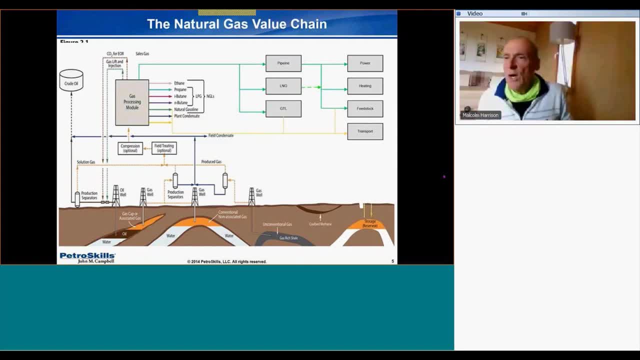 two slowly. Question number two is how many of you would be interested in in coming along to part two of the series and talking a little more about, Well, the bits that I didn't talk about, the bits I didn't talk about. I'm trying not. 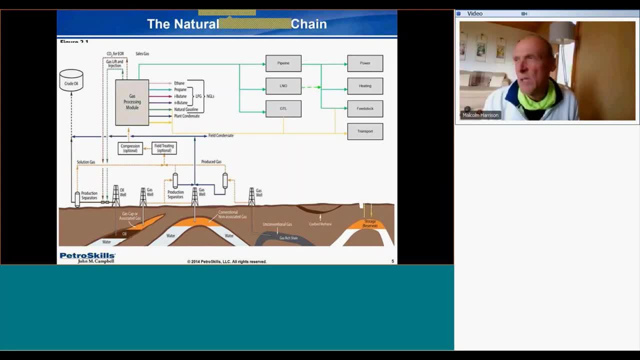 to use the words a bit. that was was the impact of availability and the impact of efficiency, And now I've given away the secret, but the the big downside to both wind and solar, obviously, is that they don't work when the sun's not shining and wind's not blowing. 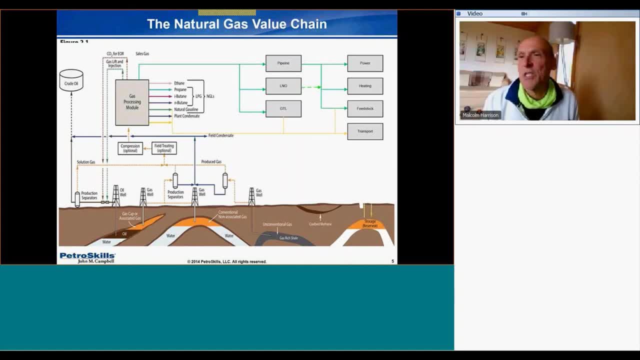 The, the, the solar panel actually produces a capacity of less than 20% of the time. But so so back to ticks Again. but would you be so kind as to check if you'd be interested in steps two, three. 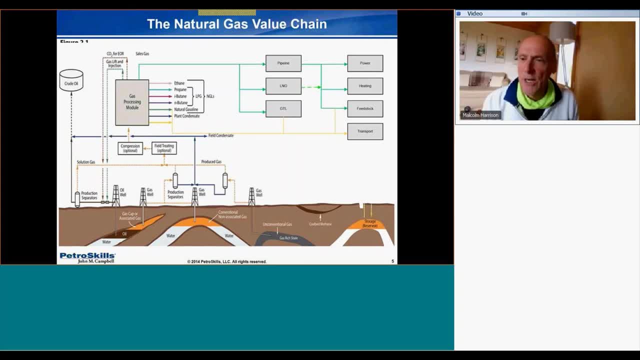 four and five of the series. could you click your buttons And we're getting far better at voting And then, if you do come back again, I promise I'll get far better at presenting. So that play that successfully avoided me asking answering questions for a few minutes. 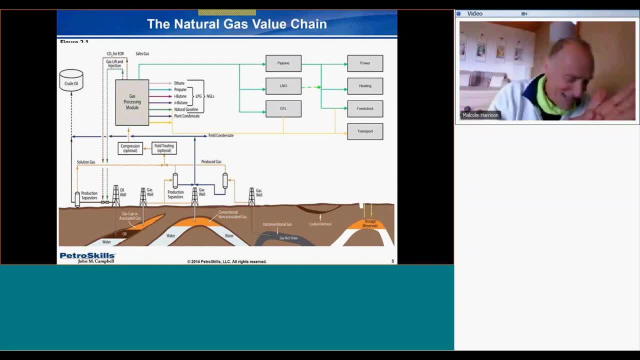 but we've got anything, anything more I can help with? Yeah, I've got. I've got a couple more here. So this one asks in short, if that's possible, I'll add parenthetically: How can we economize GTL processes refinery with the current supply chain of oil and gas? 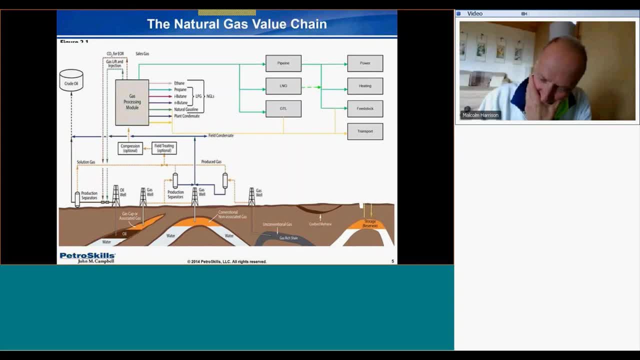 How can we economize GTL processes? This is a personal view. This is a personal view I. I don't think I would try. I realize in saying that there'll be people who are engaged in in doing this very task that will rush to disagree. 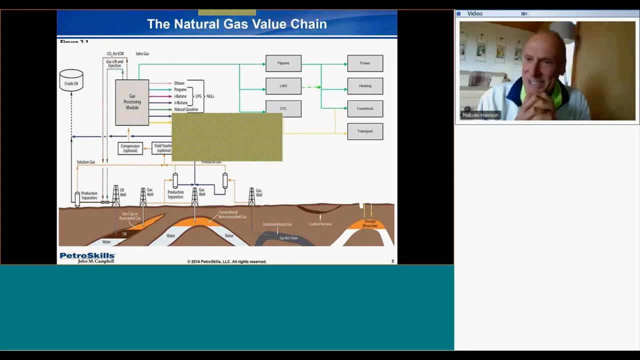 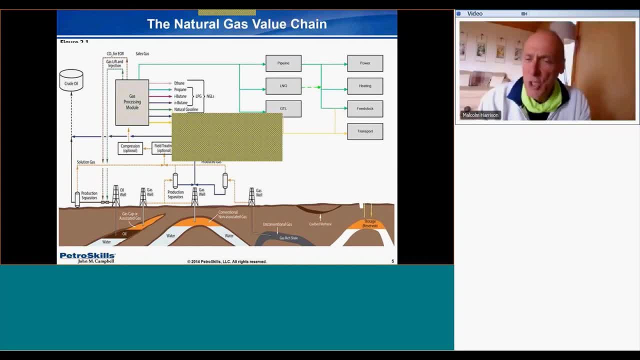 The capital cost is high, The efficiency is, the efficiency is low. There are four GTL plants in the world at the moment: One in Qatar, which which is there more for strategic and portfolio reasons than anything else, A number in South Africa. 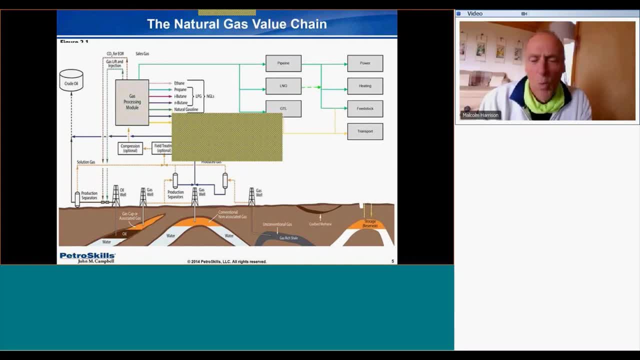 I think we know why. why they are there: One in Nigeria. Very few of the decisions that are made in Nigeria are made for strictly commercial reasons- And then one in Malaysia, which was a trial. I don't I don't think other than niche applications. 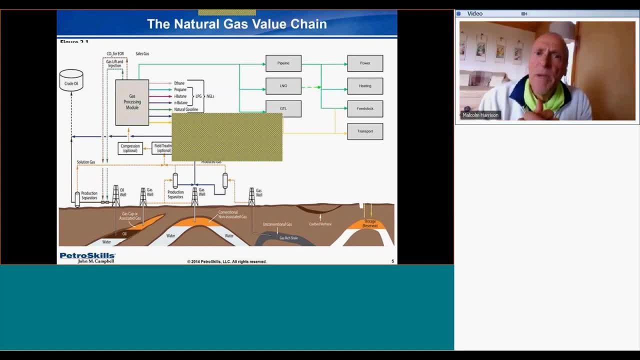 I don't think GTL is ever going to be mainstream And people used to say that about LNG And clearly it is. It is now, But I many people online will know this already. But I think Uzbekistan- actually Uzbekistan is- is famous in the world for being this. this. this could come up in a quiz as being the only country in the world that is doubly landlocked, ie it has two countries on every border between it and the ocean. It also has very large reserves of gas, but no way of getting it to the market. 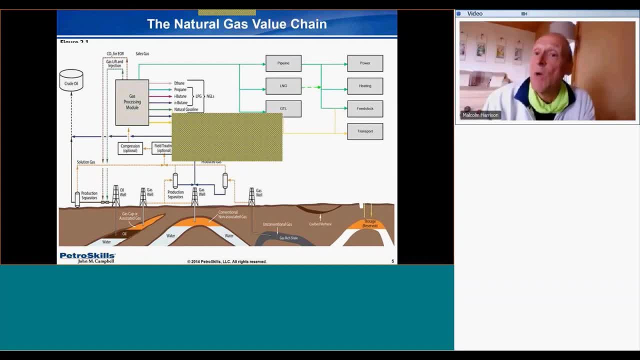 So you might have niche applications Like that, where what they're doing in Uzbekistan is saying: well, we can't, we can't use this gas, They're going to close the shop in 2050.. So we're going to put a GTL plant in. 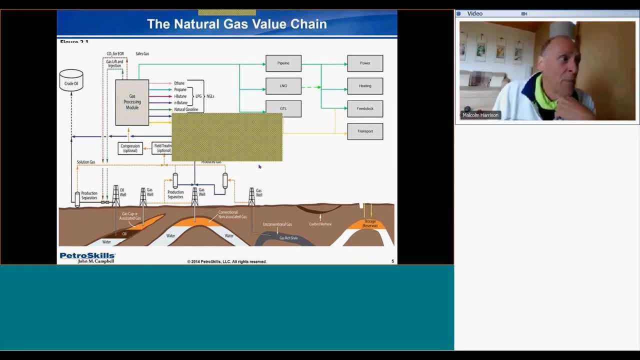 We're going to generate gasoline and we use it in the local market And maybe there'll be a few other niche applications like that. But I don't, I, I, the fundamentals with GTL are just are never going to, are never going to take it to be mainstream. 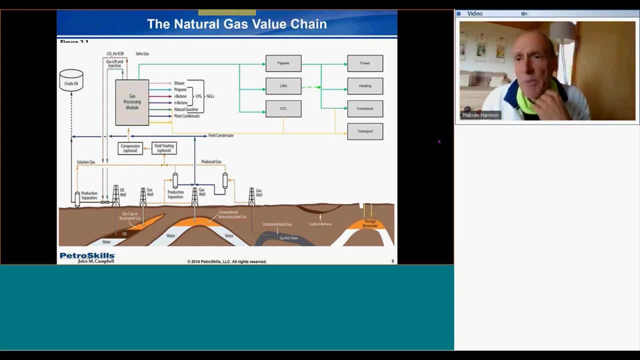 And I. it's a shame we can't hold a discussion, Because I think there are lots of people out there who disagree with me, but it's such my personal view, All right. And then the next question asks: what is blue ammonia recently shipped to Japan from Aramco. 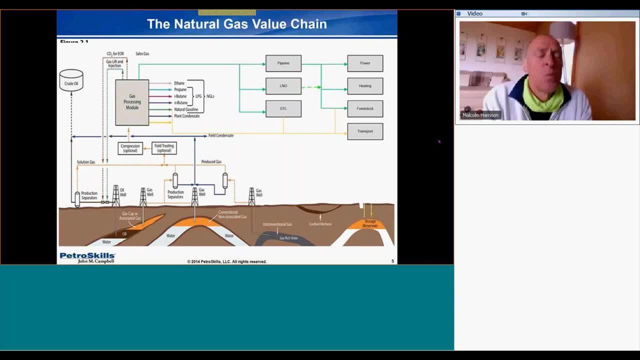 And how does it fare as fuel for power generation? Oh, I don't know. Do you know? can I take that one on board? And if, if, if, the person who asked it and anybody else who's interested wants to drop me an email. 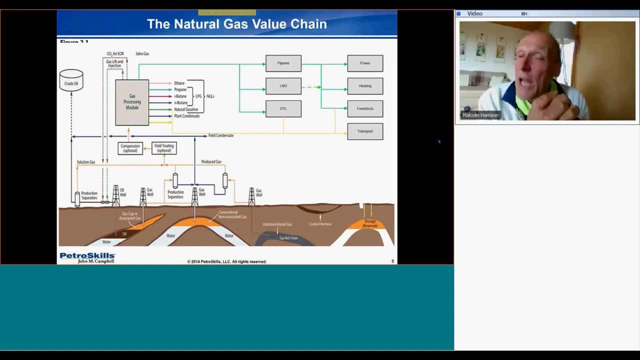 that that needs. that needs a bit of a bit of contemplation. It's something I'd like to do because I would very much like to know the answer, But at the moment I don't. But I'm happy to take it as an action if you'd like me to dig into it and get back to you. 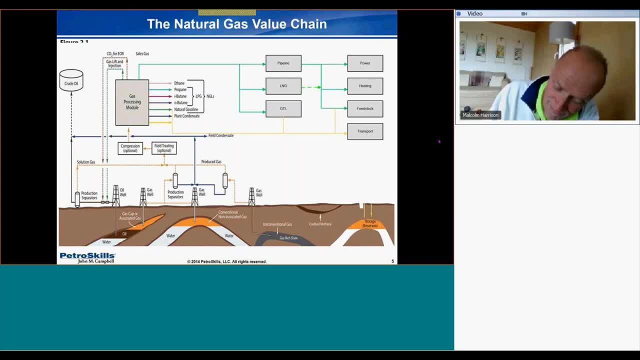 Yep, fair enough, And then that's it for the questions. There were a handful of questions asking your thoughts on renewables And various bits of technology there, So I will use that as a bit of a tease and an advertisement for the next section. 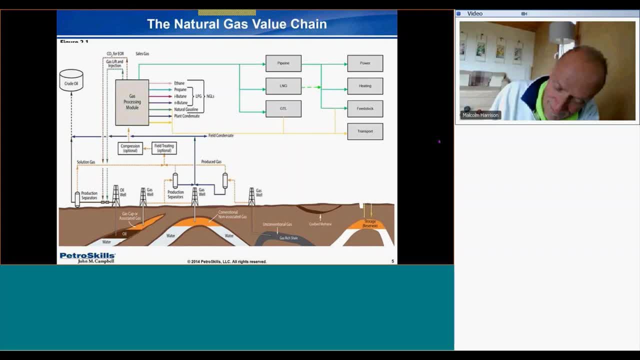 We will collect those comments and get those to you So we can make sure that you're covering that stuff in the subsequent renewables conversations. So thank you everybody for for the questions for the discussion. Malcolm, thank you very much for answering.